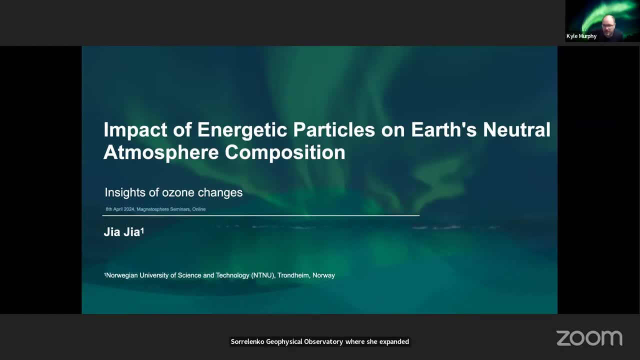 research to the polar middle atmosphere and space-weather coupling. Since 2021,, she's been based in Trondheim, Norway, at NTNU's the Norwegian University of Science and Technology Atmospheric Dynamics Group, where she has been focused on understanding how energetic particle precipitation 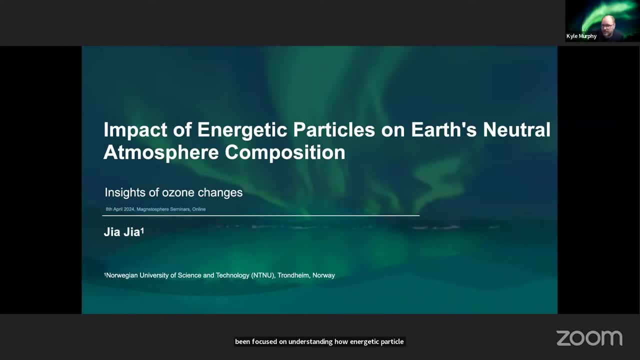 induces chemical changes coupled with the polar vortex and wave propagation using satellite data, reanalysis data and model simulations. With that, if you would like to take it away today. Thank you, Kyle. Hi everyone, And so today I'm going to talk about the impact. 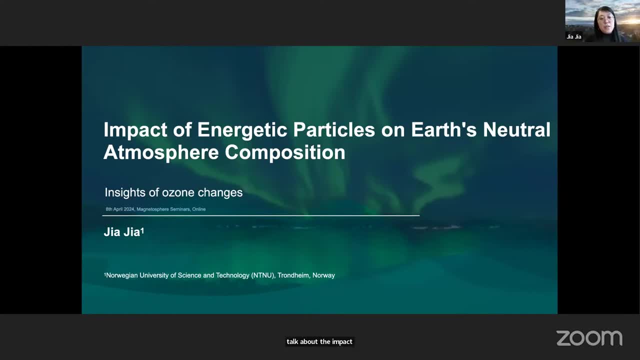 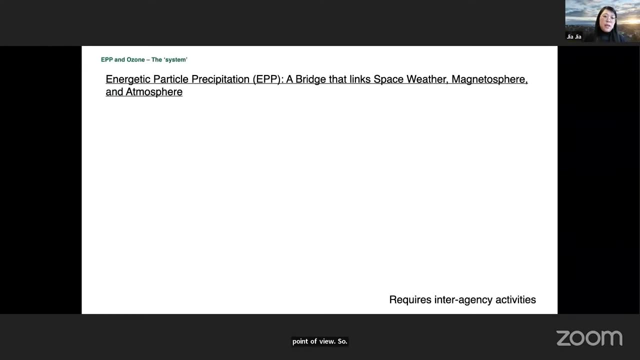 of energetic particle precipitation on the atmosphere point of view. So I start with introducing you with energetic particle precipitation And this kind of phenomenon. to my understanding, it's a bridge that links space, weather, magnetosphere and atmosphere, So it's a big system. 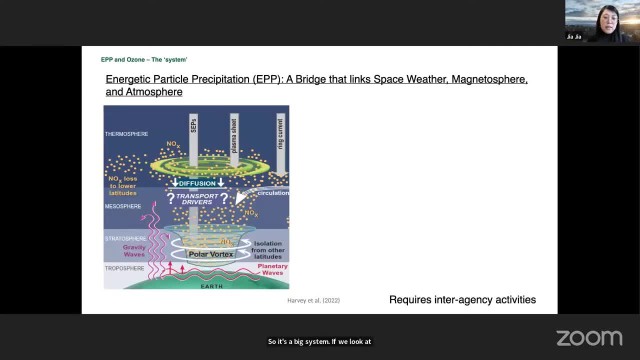 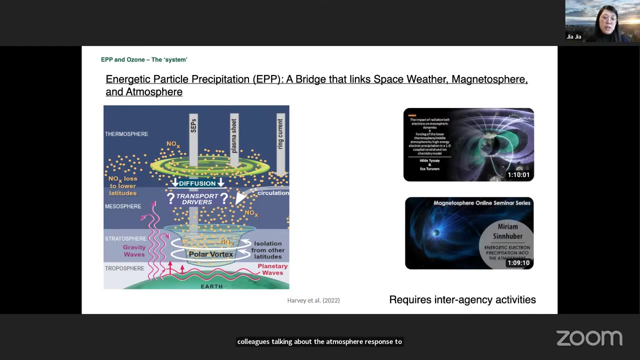 If we look at atmosphere itself- and this is a whole system- that looks very complex, and a lot of things have been going on in this seminar. Actually, there have been several of my colleagues talking about the atmosphere response to this EPP event. So, since I'm the fourth person to give this kind of talk, I'm thinking like what? 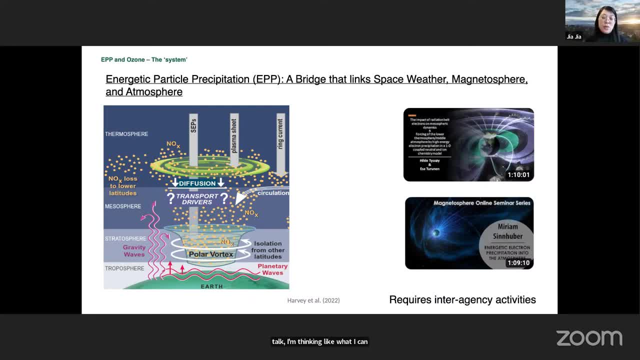 I can bring something new to this seminar. So I decided to go from the perspective of ozone. Not only that I've been studying ozone for a while, but also, like ozone is one of the critical links that that makes everything runny. But I think, don't worry, I will start to talk about the basics of this story. 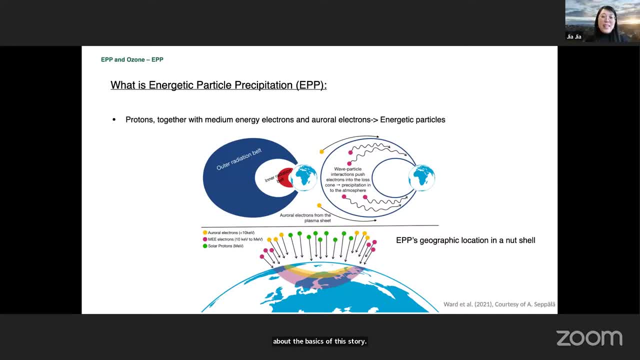 I will not jump directly to ozone. So the basic story is like so, first of all, what is energetic particle precipitation? So, in case there's any astrophysicist here, So just to say that our energetic particles are the protons electrons with tens of ke1. 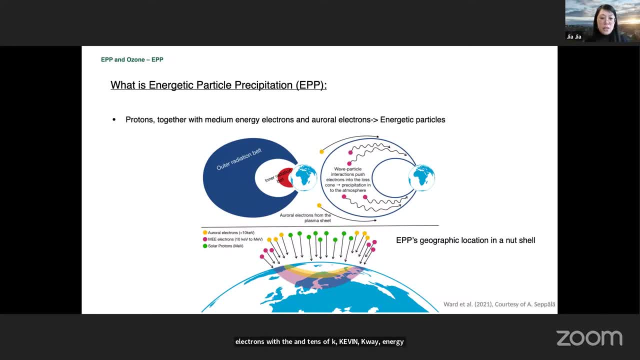 Ke1 energy and, to me, energy. So so, compared to astrophysics view, this is not really super energetic, But these are the ones that matters in the atmosphere. So I really love this, this picture, because it gives you a general view of the 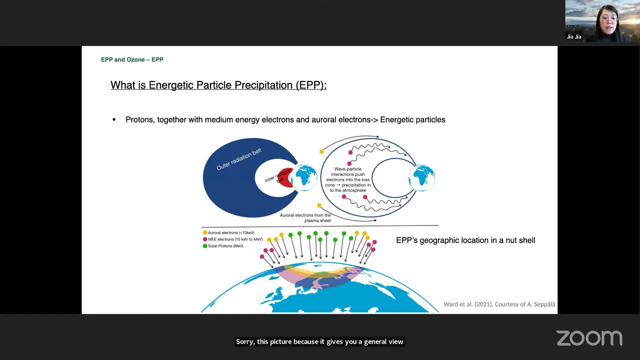 geographic location of where these particles are working on. So, as you can see that the green ones are the solar protons, They works, the energetic they inject directly to the whole polar cap area, and the yellow ones- And the yellow ones- are the aurora electrons. 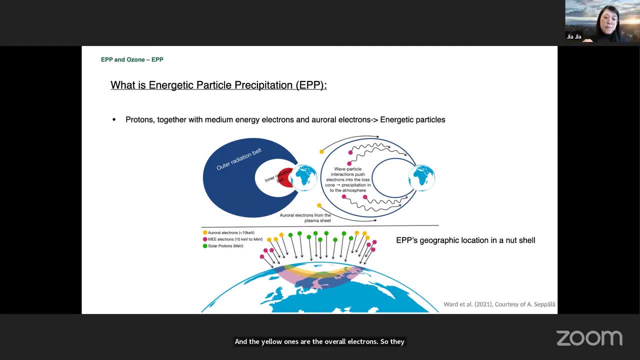 So they come in as aurora, aurora areas in the in the high latitudes and the middle energy electrons. they are the one that you guys are familiar with with the magnetosphere interaction in the outer radiation belt And they gain a little bit higher energy. 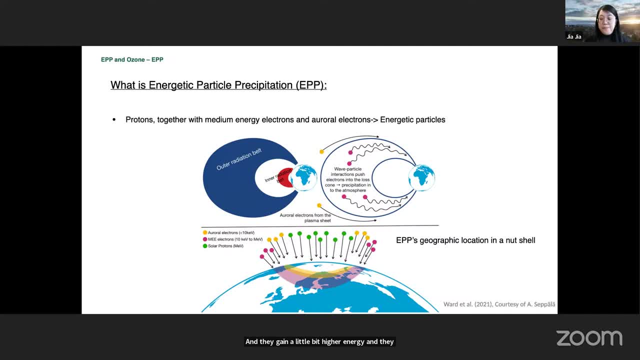 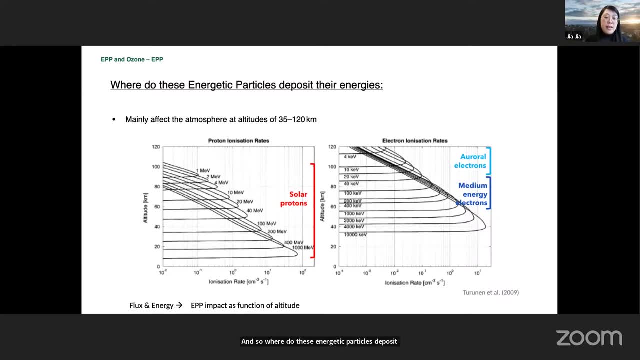 and they are precipitating more of the south of the aurora aurora area. And so where do these energetic particles deposit their energies? They are energy levels, of course, And the higher energy they are, the deeper they can go into. This is a nutshell about where these electrons and protons are reaching. 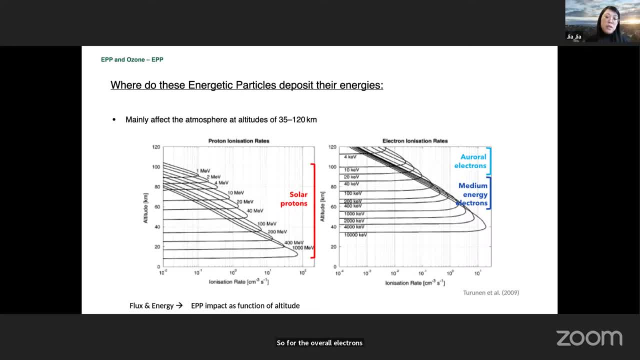 So for the aurora electrons it goes in the atmosphere view. This is more like a thermosphere And the energies with the higher powers they are working in, in our view more of a mass sphere, so-called. And for the solar protons it goes from the upper side until the lower atmosphere. 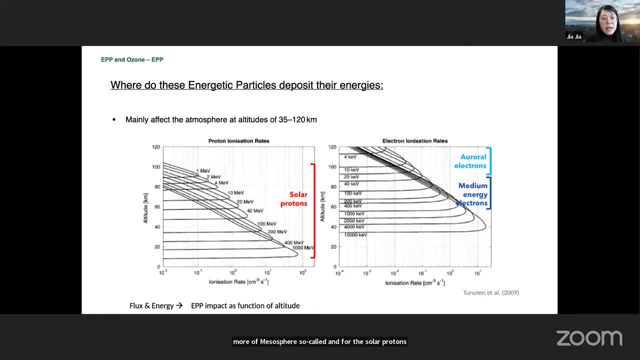 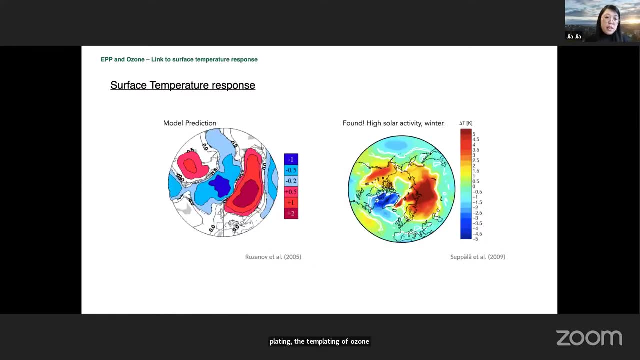 which is the lower stratosphere. Now the whole story, wrap it up, is that this kind of event that depletes ozone. So why we care about depleting of ozone? And one of the exciting milestones of this energetic particle precipitation is 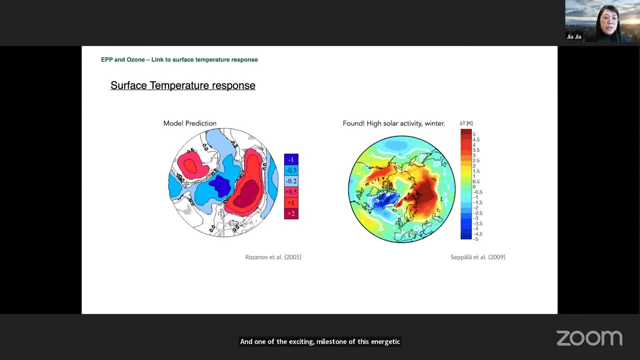 that we have found the surface temperature response to these energetic particles. So it was first predicted in the model in 2005,. as you see in the left side- I don't think my cursor works So I'll just describe it- And on the right side is what we have found in the real data. 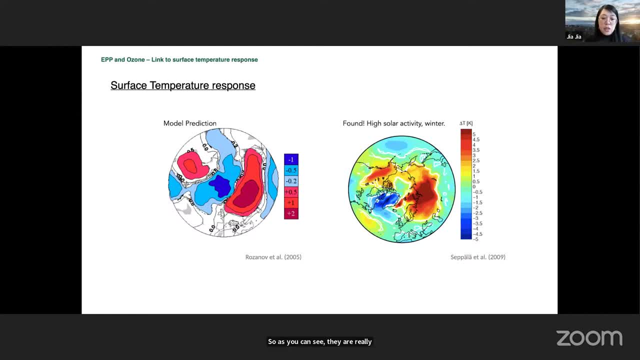 So, as you can see, they are really consistent, And the energy, the temperature response, is kind of like high. Now the question is why? So we were trying to understand it, And the ozone is one of the critical links that could bring us there. 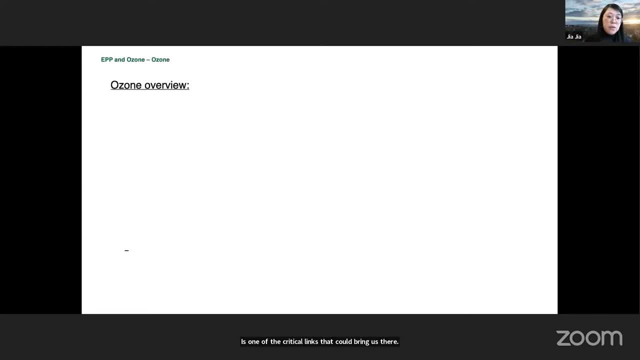 So now, what is ozone? I will give you an overview to talk about ozone. So the whole atmosphere, the ozone is created through this one link, which is atomic oxygen plus O2. with some collations, you will form ozone. The question in different layers is where this atomic oxygen is coming from. 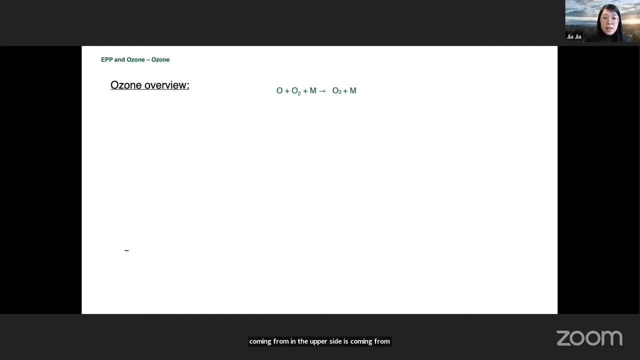 In the upper side is coming from the molecular oxygen In the troposphere. another story is coming from NO2.. But in general the O and O2 formation is the key point of forming ozone And now there are different balances in this whole atmosphere. 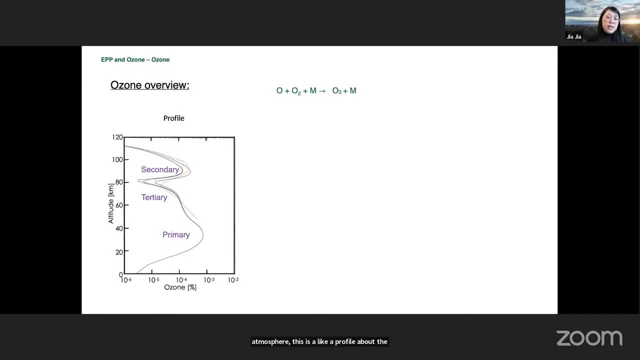 This is like a profile about the ozone And you can see that it has three big layers. The primary ozone layer is on the bottom is the one that we know as the ozone hole, where the ozone layer stays as a critical part to protect us from UV radiation. 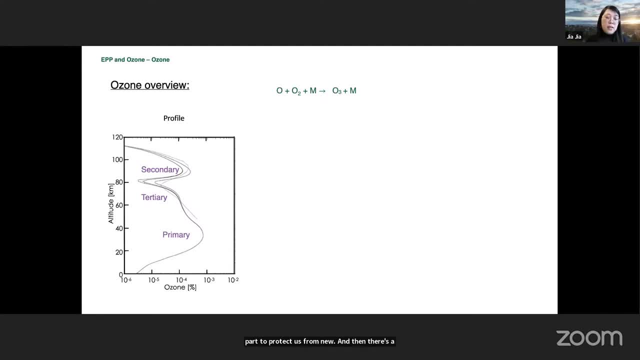 And then there's a permanent secondary ozone layer sitting in the thermosphere- lower mesosphere, Sorry so, mesosphere, lower thermosphere, And this is also a permanent layer. And the third one in the middle is a tertiary ozone, And this one comes and goes, depends on different occasions. 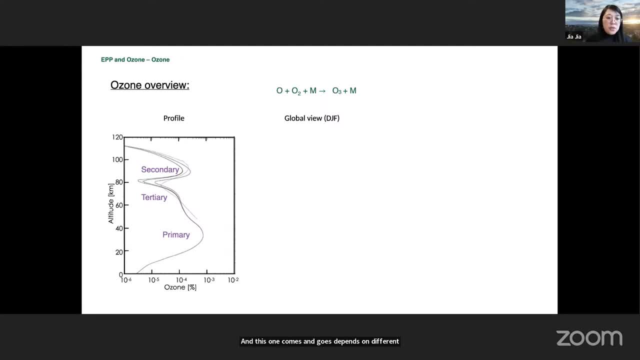 So to give you a global view, since we care about more winter conditions, I would jump directly to the winter. So this is a global view of ozone data. And so now you have from the southern pole to the northern pole, left to right, and then, with the profile, look. 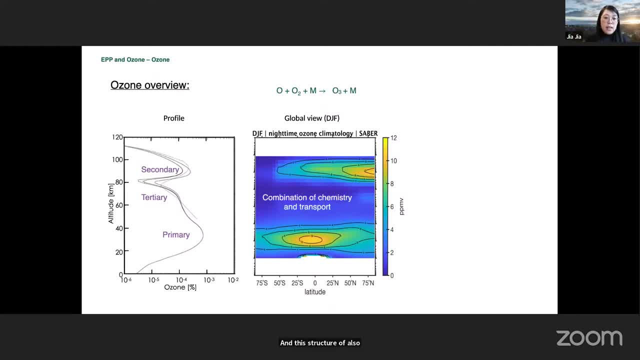 And this structure of ozone distribution is a result of chemistry and transport. So there is creation of ozone, deflation of ozone, doing the chemical things. But also remember our atmosphere is running around dynamically. So to understand which one plays a more role, we can look at the lifetime of these compositions. 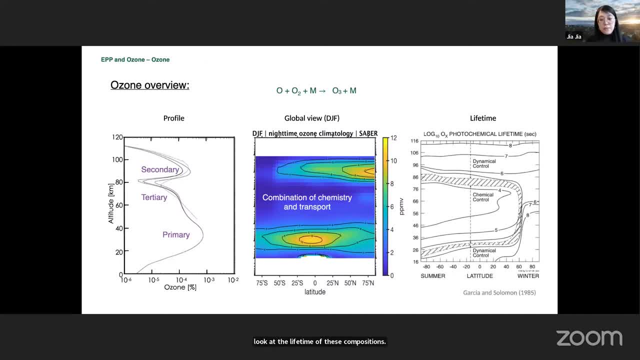 So for ozone the lifetime looks like this, And again you have the summer and winter and the whole global view with the altitude. So this is lifetime of seconds with the logarithm. So to make your life easier here, this number four means it has hours of lifetime. 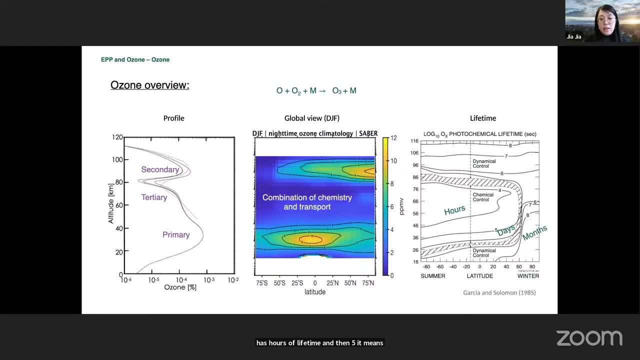 And then five, it means already days of lifetime, And then when you have six, seven, eight, it means it comes to the month, So which means that it can be transported around with how the air circulation goes. So on the top you will notice that it's also dynamic control. 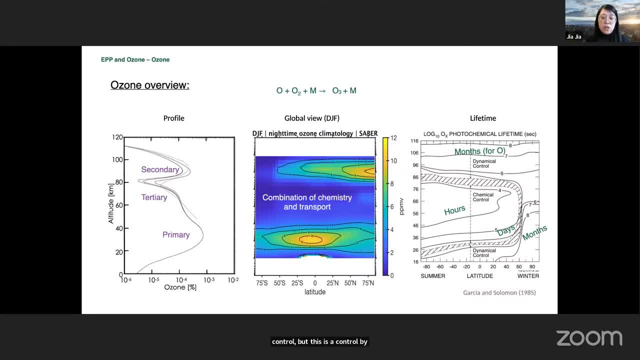 But this is a control by the source of ozone, which is atomic oxygen. Ozone there itself has a very short lifetime, but it's very sensitive to atomic oxygen, which is very long lived there. So it can be understand as like reflecting of dynamic control as well. 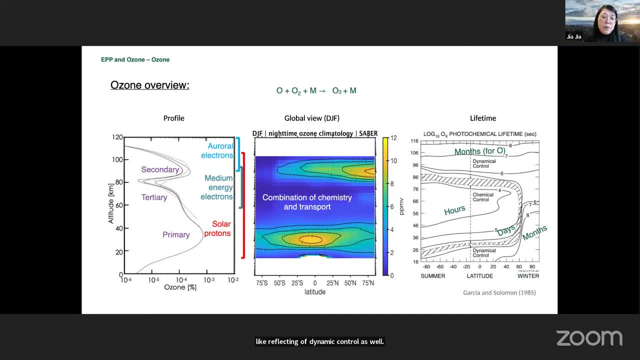 Okay, Now, when you have the EPP comes in the energetic particles in the polar region. what we focus is then the summer pool and winter pool, And now you notice in the summer pool, actually between these two, this chemistry that dominates well in the winter pool. 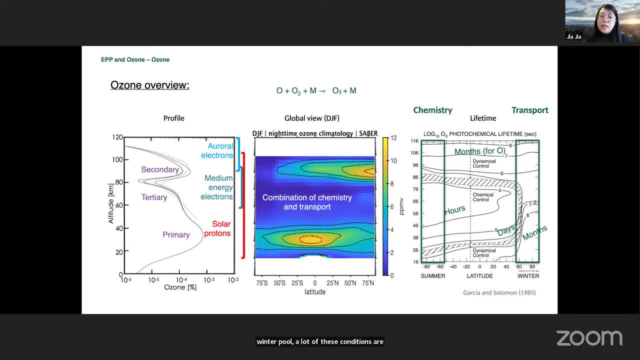 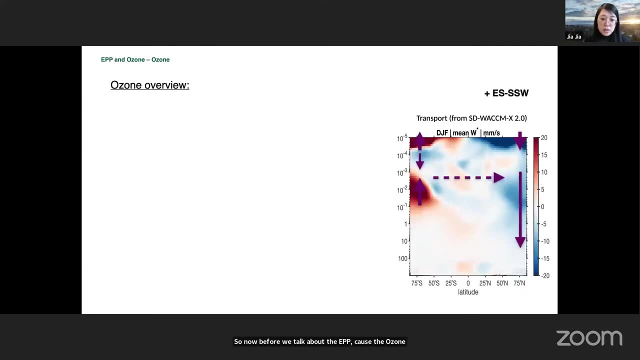 a lot of these conditions are transport. It doesn't mean that chemistry is not important, But just to tell you that transport also plays a very critical role in this area. So now, before we talk about the EPP caused the ozone variations, let's take a look about transport. 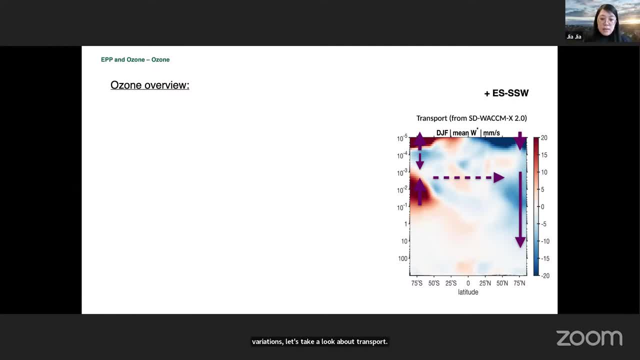 So this is from a model called Wacom X And it gives us how the ozone, how the atmosphere moves, And this is the vertical movement. So if you look at the blue colors, that means it's going down And the red ones means it goes up. 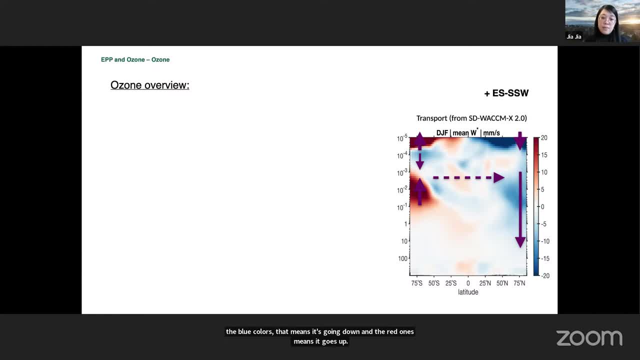 So what you can see is that in the summer hemisphere you have this lower branches that is going up and then across the whole atmosphere globally and going to the winter pool and going downward, And that is caused by the gravity wave drag which is filtered by this special wind wall which is called polar vortex. 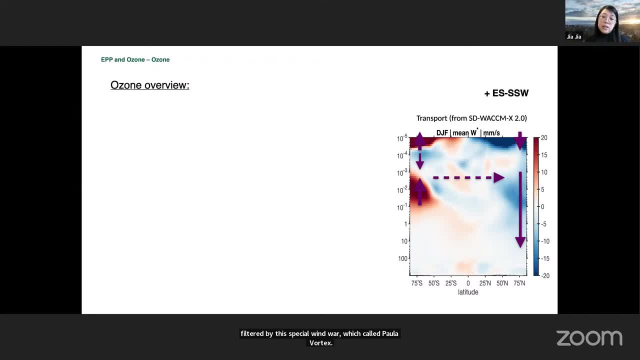 And it forms only in wintertime. So that creates this global circulation And now you notice that in wintertime that there is a downward transport in the polar regions which will play a critical role when we talk about EPP and the atmosphere. response. Now in the polar region. the other thing that moves the air up and down is the so-called elevated stratopause, sudden stratus warming, Just to make your life easy. it means some event that will drag more of the atmosphere air into the lower part. 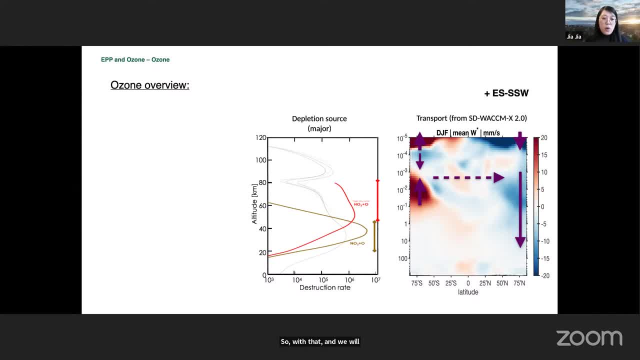 So with that- and we will look at what kind of depletion source does ozone have- we know that the creation is always O and O2.. So when we talk about distribution, then it's like which reactions is the one that depletes it? 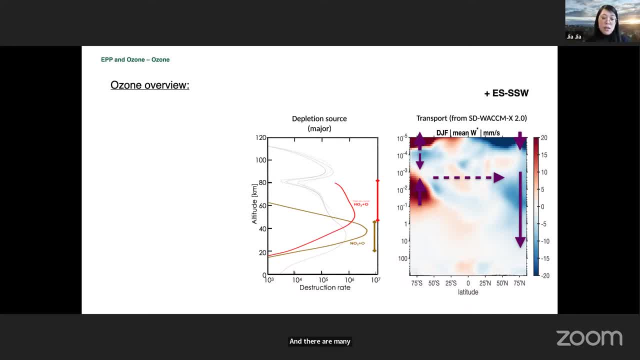 And there are many depletions going on. So just to make it simple, so there are different areas, like there's one trace gas, one of these reactions that dominates. So in the mesosphere it's HOX and in the stratosphere that's NOX. 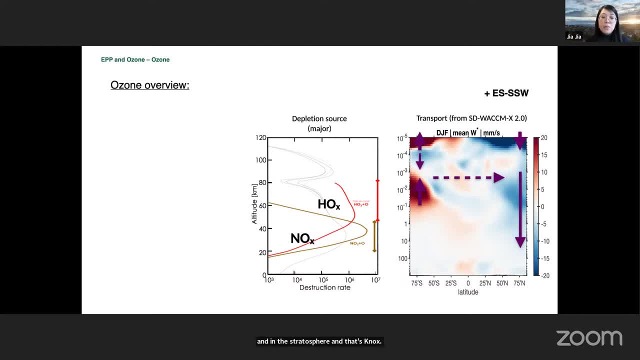 So they are the dominating ones. There's many other things, but those are the one that mainly controls it, And how they deplete ozone is from the so-called catalytic reactions. So the net will form O plus O3 to deplete ozone. 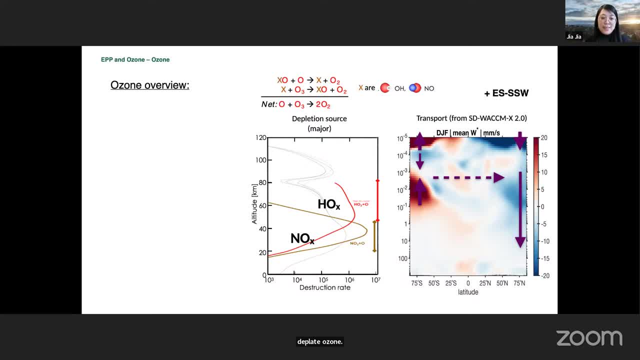 Now, if you remember, we have a secondary ozone layer- It's about there- And the upper side. actually, none of HOX and NOX plays a role. The main depletion is atomic hydrogen. So if some of you are familiar with airglow, 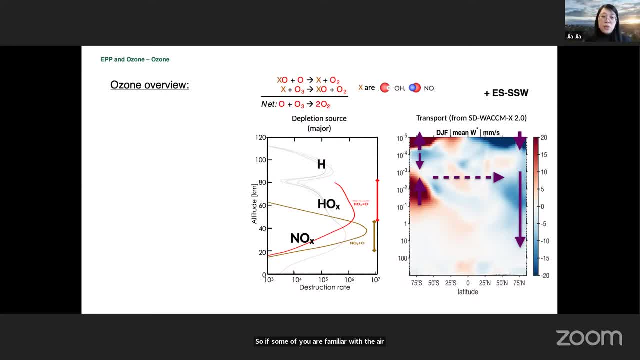 so this atomic hydrogen and ozone reaction are the source of airglow in this area. So why the ozone is important is that it is a radiative effect. It's very strong. So what you see here with the purple lines are the, the radiative effect of the whole atmosphere with all the compositions. 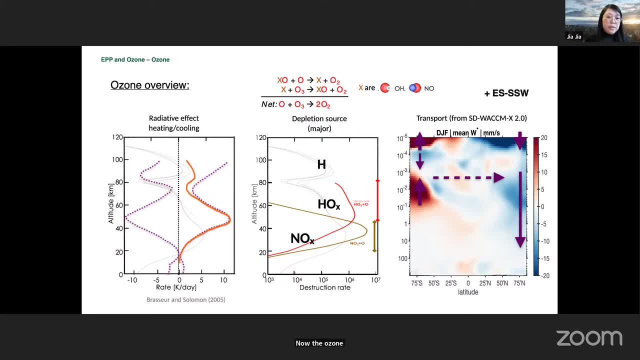 Now the ozone when it goes for radiative warming, and these orange lines tells you how much is coming from ozone. So it's a dominating radiative warming source And it also emits energy. So it also gives you the so-called radiative cooling through the longer wavelength and it looks like this: 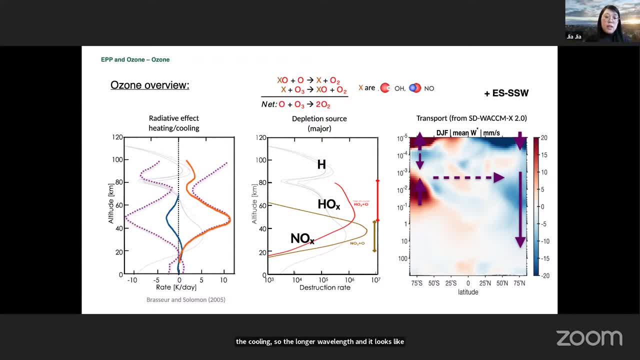 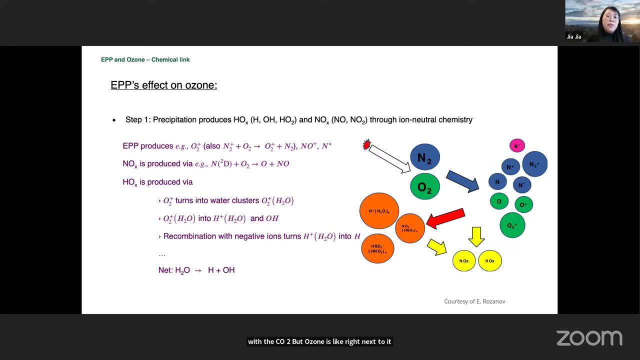 So the rest of things are what we are familiar with: the CO2.. But ozone is like right next to it. OK, now, if it comes to the EPP's effect on ozone, I will give you like a very, very simple two steps. 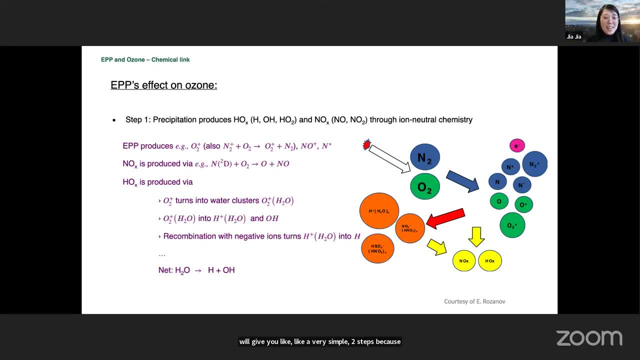 because, like our colleagues has talked about it a lot in the talks before, So I don't want to repeat it. Step one is this: energetic particle presentations will trigger this so-called iron neutral chemistry And then they will produce HOX and NOX through all these chain links I linked below. 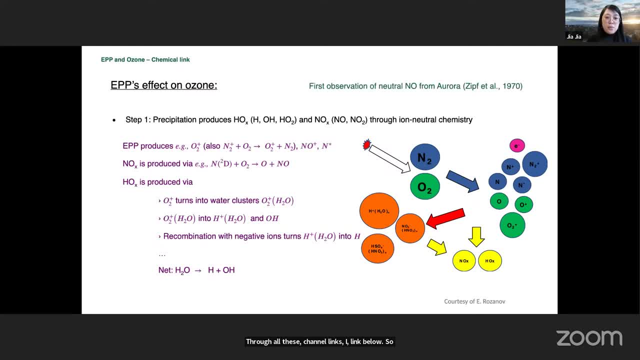 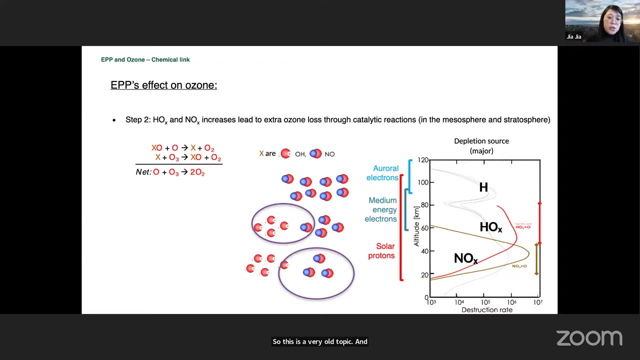 So there is one fun fact: that actually the first observation of the NO being produced from the energetic particles presentation is reported in 1970 already. So this is a very old topic. And then stop two is that those increased NOX and HOX, as we talked before. 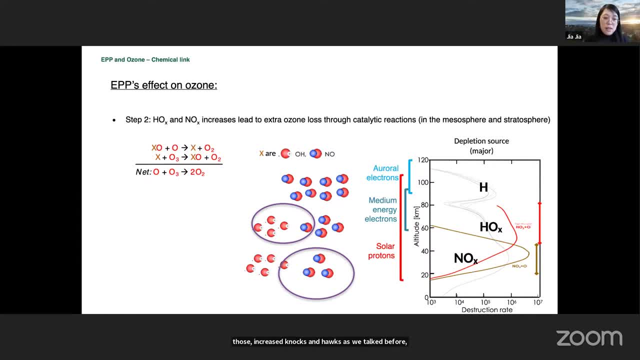 since they are the dominating eater of ozone, it will deplete ozone. So now we know that one of them takes care of one layer, So there's a direct effect of ozone through this creation of this compositions. But also remember we're talking about winter conditions and the air moving down. 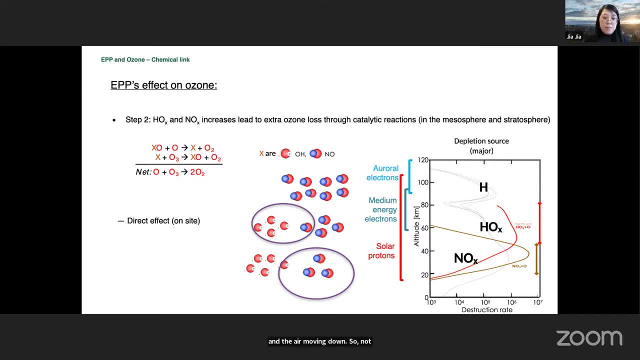 So not only ozone has a very long lifetime, but NOX also have a very long lifetime. So with the time there will be more NOX coming down, And all of this works on this primary ozone layer, So which we cares a lot. 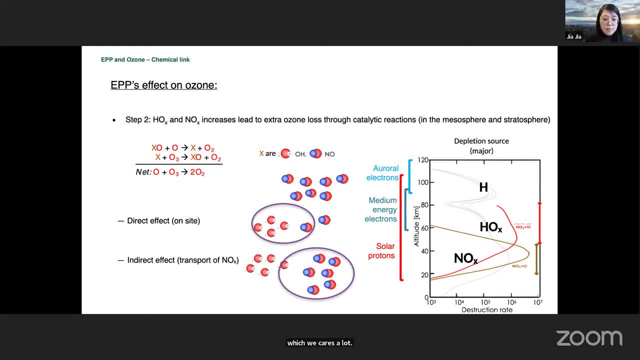 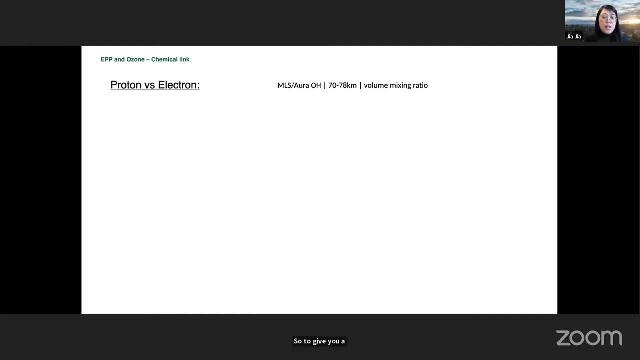 And this is called the indirect effect. So to give you a comparison or an impression about proton and electron differences, let's look at the HOX. So this is one of the HOX, which is OH from a satellite called MRS, And this is what I show here is like 70 to 78 kilometers. 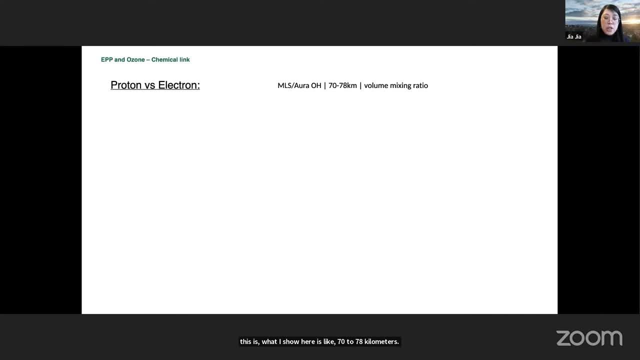 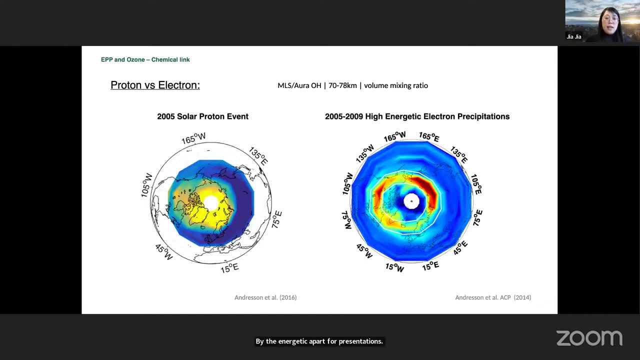 So in the mass sphere where the HOX is changed the most by the energetic particle presentations. So what you see here on the left side are from one solar proton event and on the right side from multiple energetic electron presentations. Now you see clearly that for the electrons you will 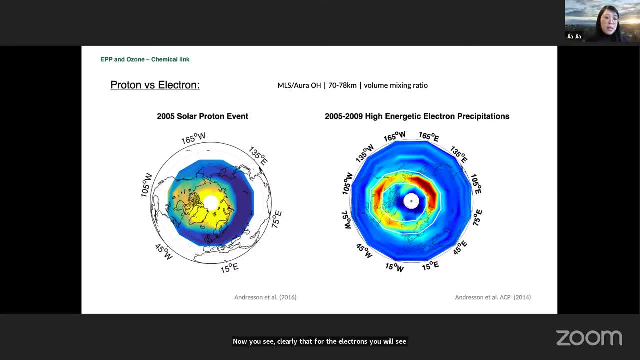 see a clear over form kind of structure. But for the solar proton event it's just a HOX that covers the whole polar cap. So on the other side the proton and electrons happens at different times. So for the solar proton event it is not very often happens. 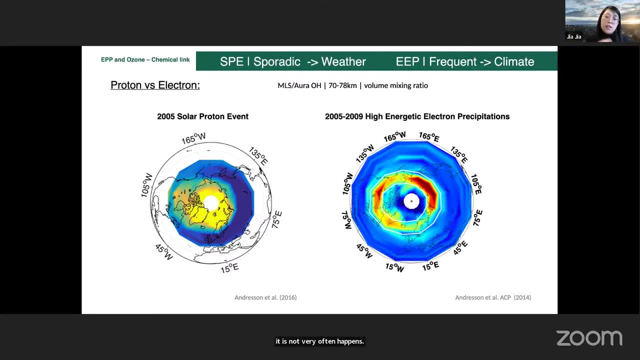 So it's more sporadic. To understand it better is if you think about weather and climate. So this is more like a weather scale things, While the electron precipitation they are very frequent and they happens every winter and like regularly. So this is more. we are talking about climate impact instead of weather. 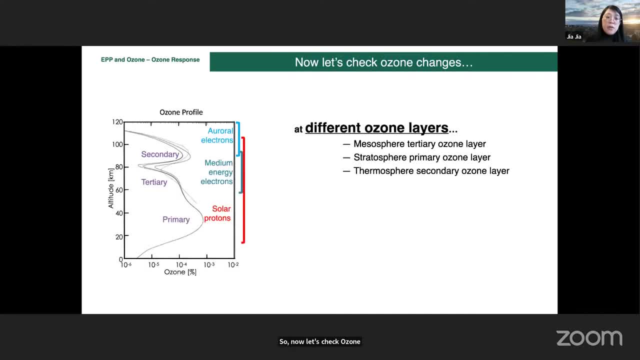 So now let's check ozone changes. I will talk about ozone changes at different ozone layers and their reaction to different events like proton events and electron events, And also I will give you like a case study and a statistic view so that you have an impression about how the ozone changes. 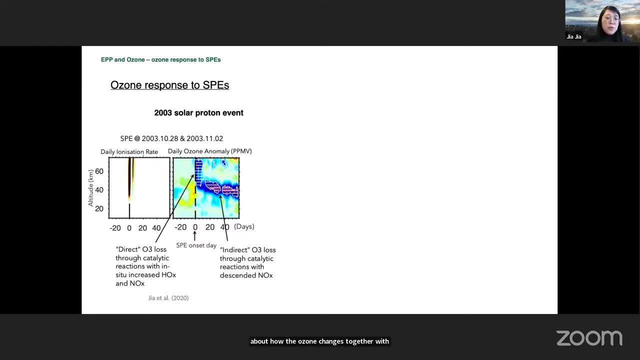 together with particle precipitation. So the first one I show you is the ozone response to solar proton event, And what I show here is a very famous solar proton event. It's the so-called Halloween event, which happened in end of October in 2003.. 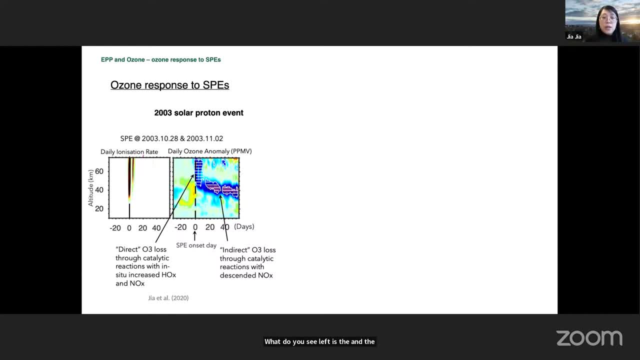 What do you see left is the ionization rate we have talking about before. So the higher energy you have, the deeper you go in. So this is one event that protons really going deep down into your stratosphere. like you can see, there is a 30 kilometer. 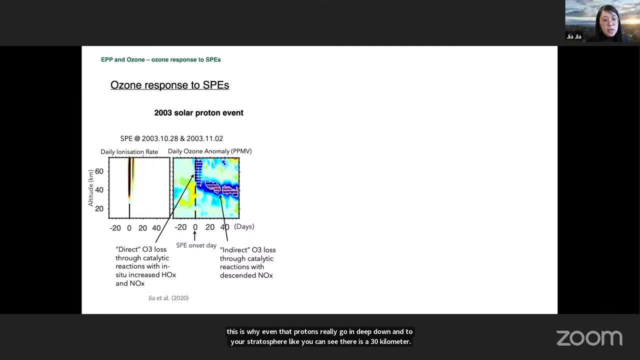 And on the right side you can see the daily ozone changes from day zero, which is what happens when this event happens- back to 30 days before and 60 days forward. Now you can see that in the stratosphere. this is really annoying that I don't have a cursor showing up. 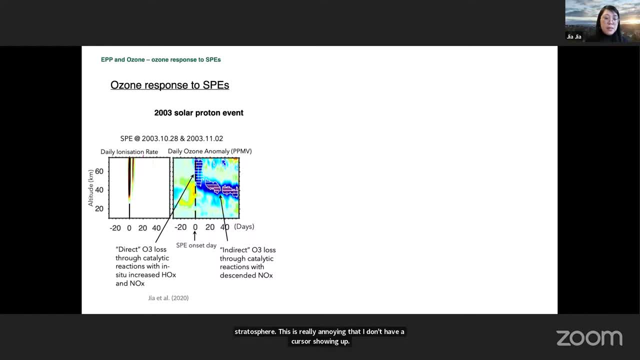 but you can see on the top part when the event really happens, you will see there is a depletion there and then there's a long tail of the ozone. depletion happens even after 60 days, like two months afterwards. That's what we talked about in direct effect. 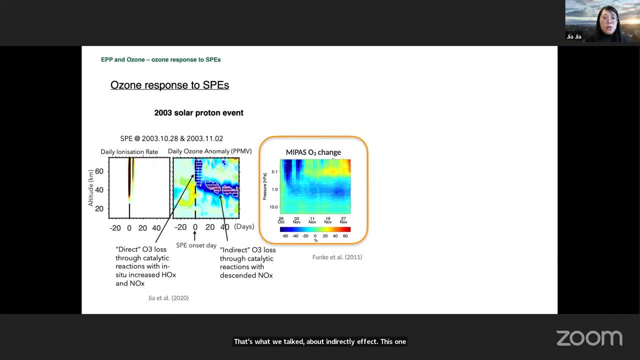 This one is from one model, but there's many observations going on This. I show you one is the satellite observation from MIPAS. It has a different scale and this is talking about percentage change, While the model I show you is like absolute value changes. 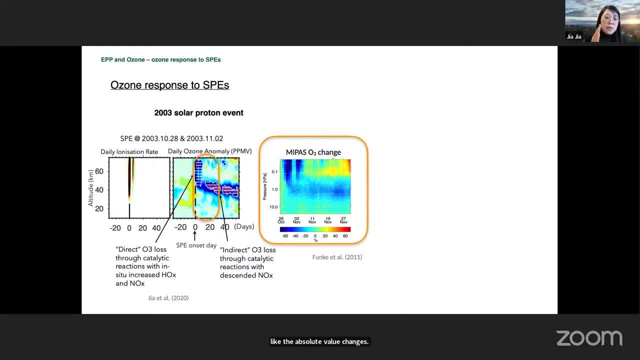 But in general you can tell that the shape is very similar and you see that the direct effects going on and then the tail continues. So this event is so famous that it has many studies before And actually back in 2004,- I have been talking about Hawks- that you see that how Hawks reacts. 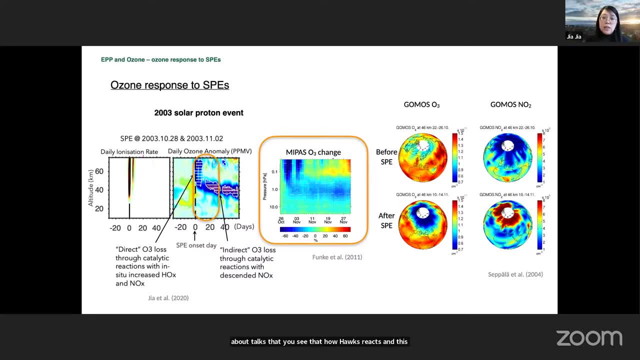 And this is an example. On the very right side you can see the NOx changes at the stratosphere. So this is a satellite observation And on the top is the before event and the bottom is after event. You see that the NOx has increased. 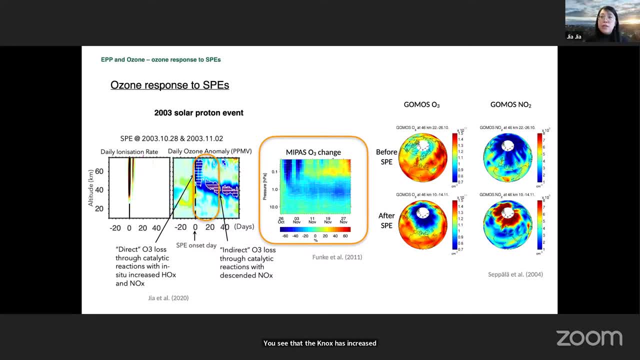 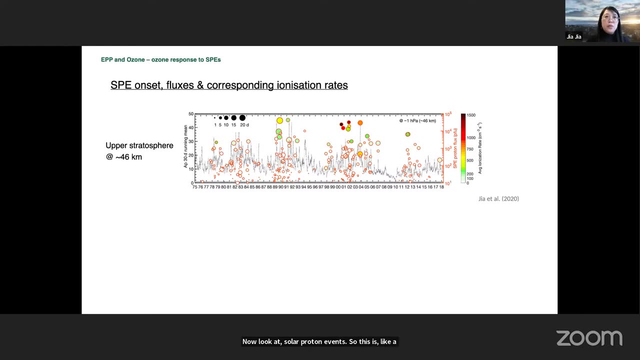 dramatically in the whole polar cap during the event, after the event And then, correspondingly, you see that ozone depletes together with it. Now look at a solar proton event. So this is like a time. This is a time series about when the solar proton event happens for 45 years. 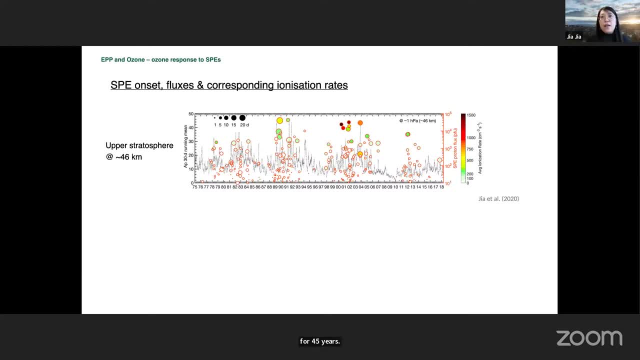 Just to give you an impression of how sporadic it is. So where I show you the colors is the ionization rate. So which means that? does this energetic particles reach this height or not? This is 46 kilometers around the upper stratosphere. 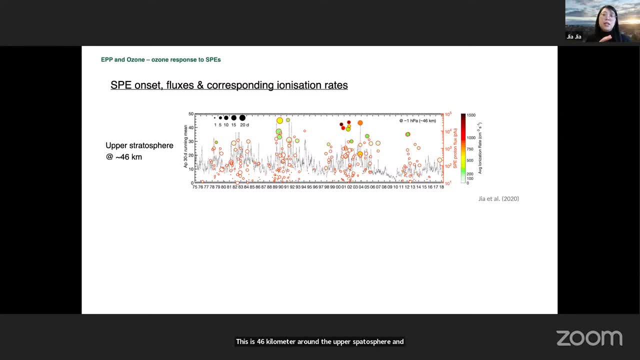 And you see that there's not many events, even like the SPE is already sporadic, And there's even less event that actually reaches to the upper stratosphere directly. So there are several of them since the so-called golden stage of satellite observations. 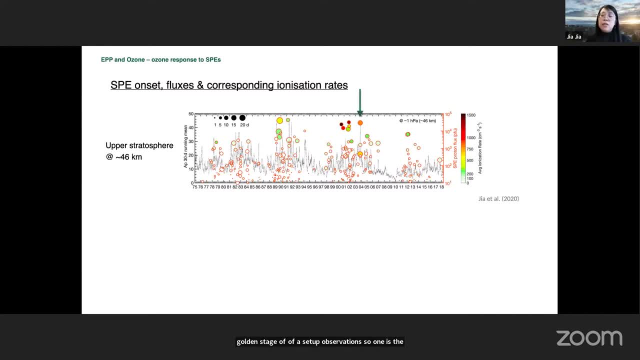 So one is the one that I said before. it's 2003 Halloween event, And there's another one, 2005 January. This is a very special case when this ionization is very hard, It's very strong, It goes deeper down. 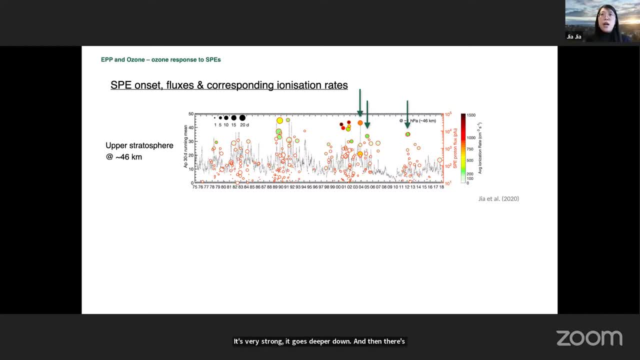 And then there's a one in 2012, January. So those are like a really countable amount, And when you move to the upper side in the mesosphere immediately, you notice that there's many more events that will work on this, on this layer, because they don't request a very high energy. 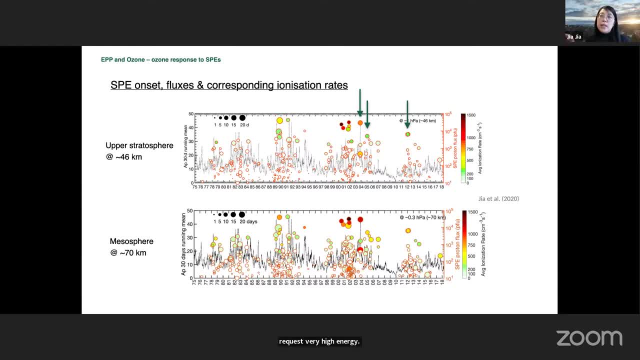 But you will also notice there's still like, if you see it's a white, the circle has no colors. that means there's no ionization going on. with this height You also see that even with the definition of solar proton events, many of those events 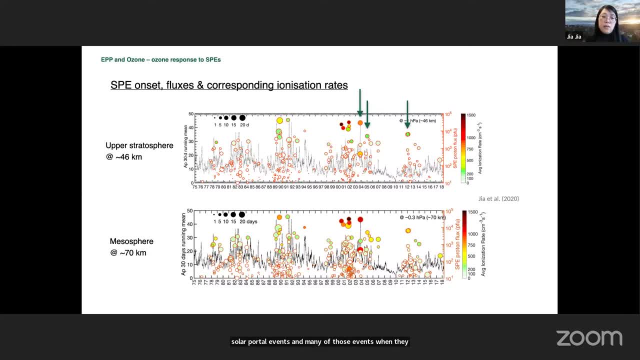 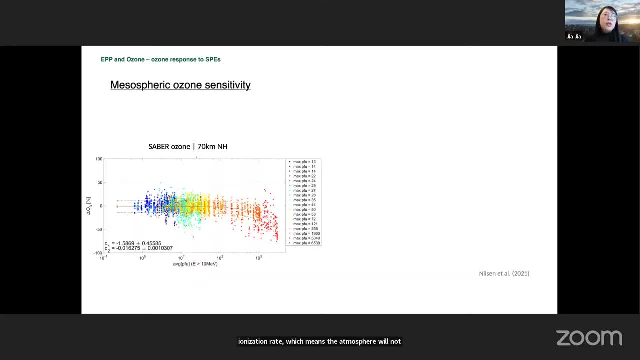 when they are very tiny, they don't really create so much ionization rate, which means the atmosphere will not respond so much on it. Now, so let's look at. this is a statistical study about mesospheric ozone sensitivity to the solar proton events. 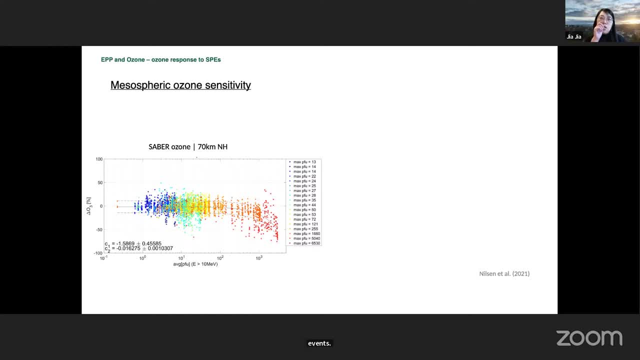 Now you see that this is using the so-called flux, So it doesn't really tell exactly like how hard the spectrum and the part particles are, but it gives you an idea like how many particles come in, So you can tell that when the fluxes are very small. 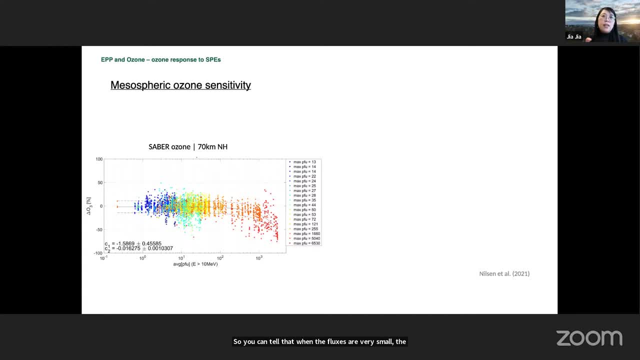 the ozone doesn't really respond so much, only when it gets harder and harder, bigger and bigger, than the ozone starts to deplace and you can see very clearly in the satellite observations. So No cursor. And so now you'll see that if you look at the x-axis, that you see that the number 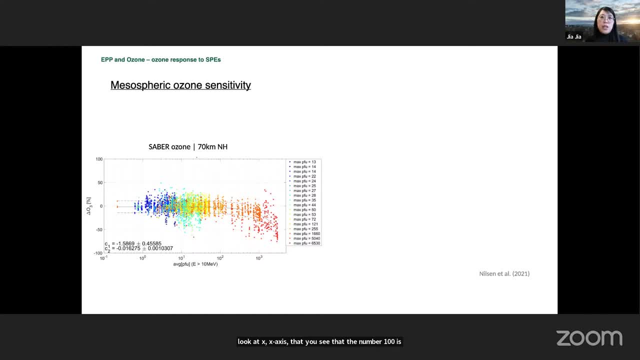 100 is the time when you start to see there's ozone depletion going on. Actually, if we take it harder time, and actually it's like around 400 fluxes that you start to see the ozone depletion. So if we do so, it's recommended in many studies that if you look at the SPE, 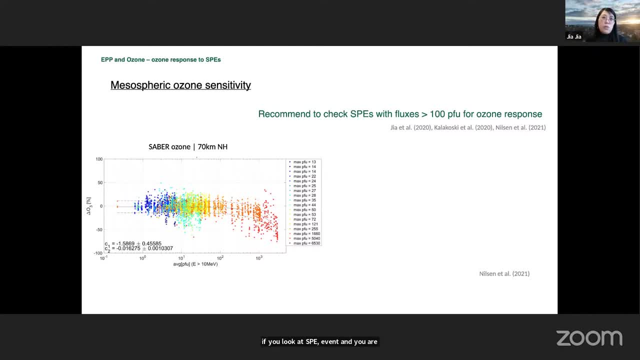 event and you are looking at, you are trying to look at the ozone response. you'd better to look at the events that with more than 100 pfu fluxes or even 400 pfu fluxes, Now, if we do a like a linear 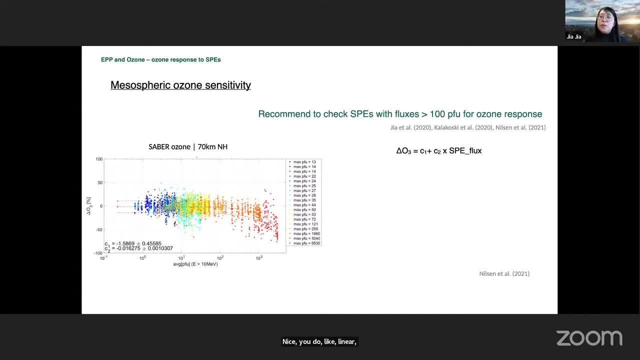 like a fitting with these kind of things, and C2 means the coefficient with the fluxes. you will get this, this profile. So now you see where the ozone response is the strongest. So it is around 70, 80 kilometer, which makes sense because that's the height where the 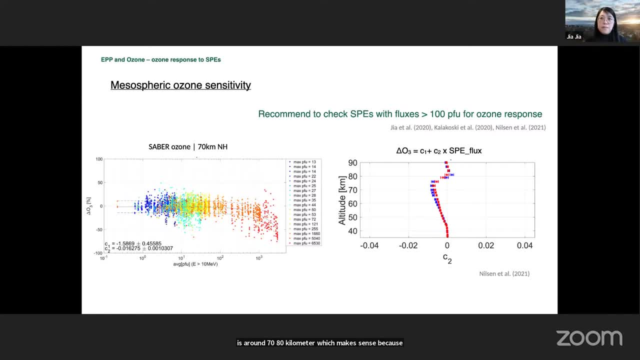 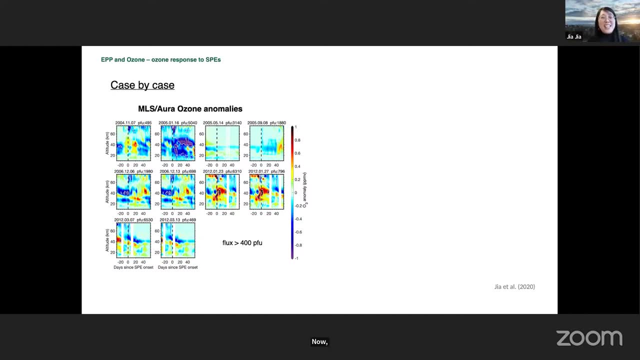 the Hawks are most sensitive to the proton events. Now, because there's not so many cases, we can actually look at the case by case. This is a similar picture with this dashed. the black lines mean the start of the event and then it continues. 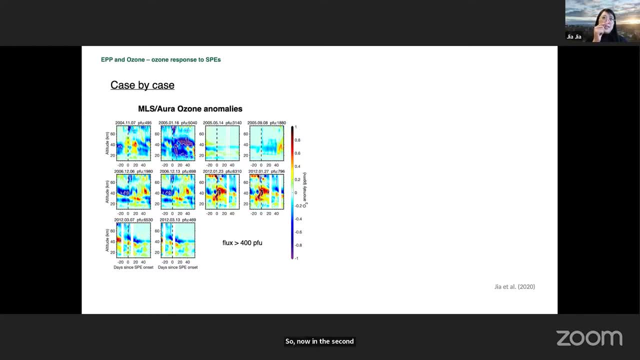 So now in the second, on the top, second panel, you will see this very big event in 2005, which I meant very typical. This is the ozone response. It has the director on the top and then it has a tail going down. 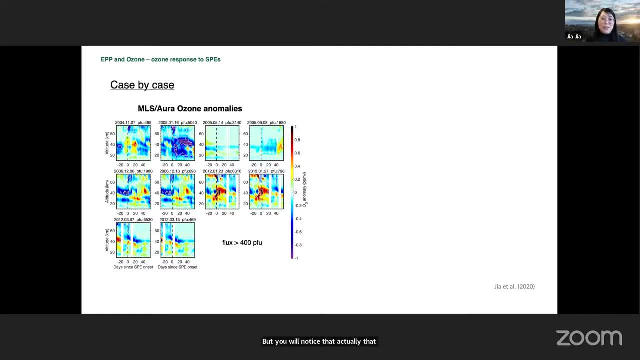 But you will notice that, actually, that not all the events are really following these nice and nice things. One reason is that, first of all, it's not really have enough energy to go there sometimes. But also, if you notice, for this events here. 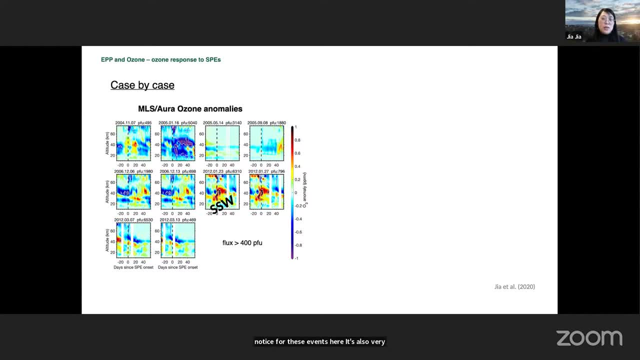 it's also a very strong event, But what you see is also enhancement instead of depletion, And that is because of the dynamic There is very strongly going on with this sudden stratus warming, which means the the, the ozone rich air from the lower latitude actually marches into this polar region. 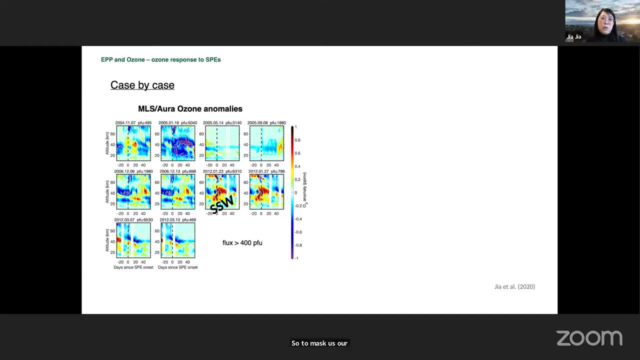 So it masks our, our effect of EPP away. And this means actually, if we really want to know what's going on statistically with these events, we actually need models, So those events influencing ozone has been reported since the 1970s. 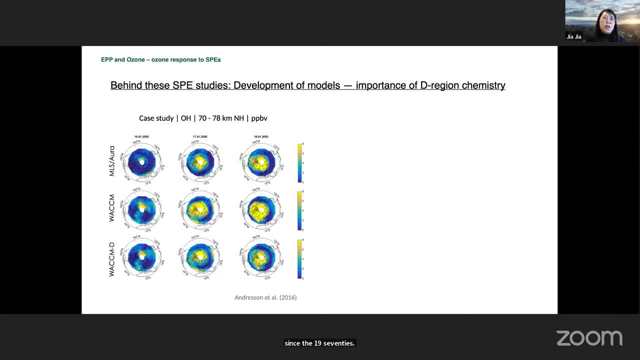 And until now. So what has been improved so far is actually development of models. So the model has been derived from the 1D model to a 3D model, But also, like we have, we have more knowledge about which chemistries plays. 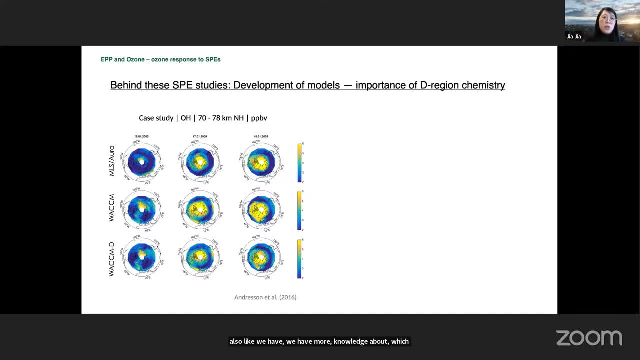 a more role besides of this HOX and NOX we are talking about. So what you see on the left on this figure is a case study again on this HOX at 70 to 80 kilometer On the top. you see this. 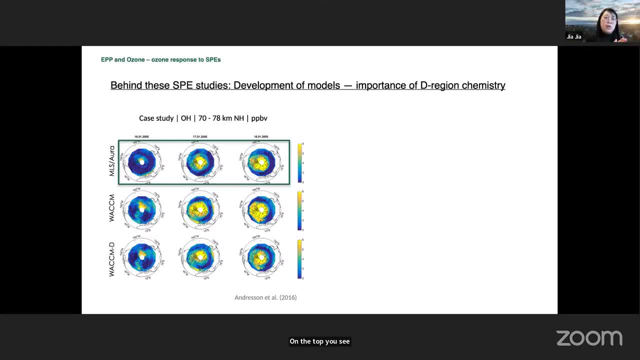 Satellite observation. This tells you. before the event it was like a dark blue colors And then suddenly the event happened. You have this white or yellow colors going on, But you will see on the second row that those is old models and you will tell. 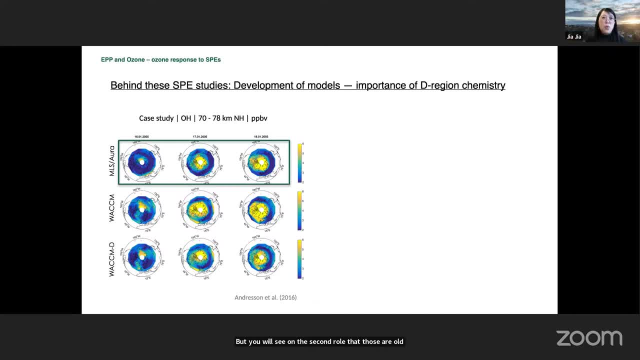 that OK. the model doesn't really catch is how much is actually overestimated Now the new model. This is an example of the improvement with these years of effort, that it goes much better Now. HOX is just the one thing. 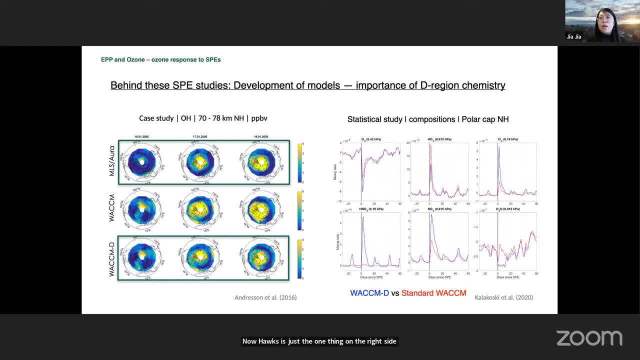 On the right side you see that there is also ozone, HOX and chlorine, which is very important, HNO3, NOX. So the blue ones are the current model, So those are all been proved that that has been better agreement with the observations. 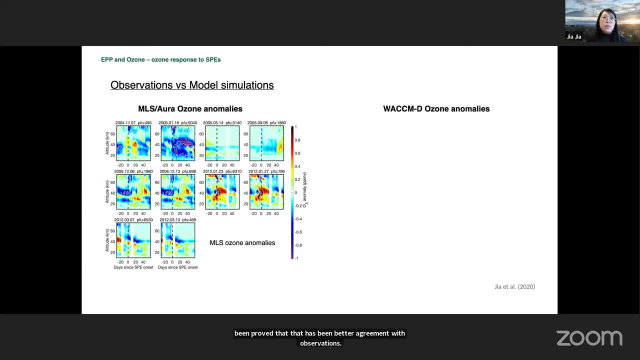 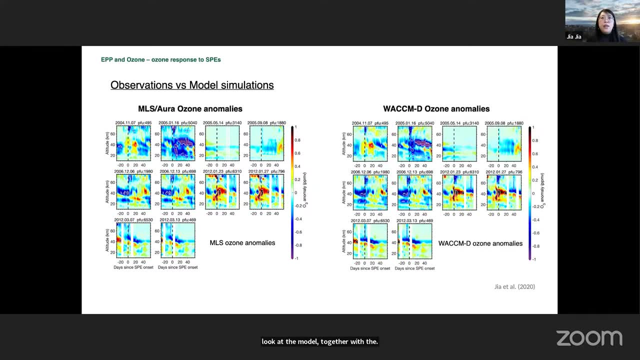 So we really have improved the model a lot. Now, if you look at the model together with the satellite observation- again on the left side is a satellite and the model on the right side- You can see that it's really reproduces what is going on with the atmosphere response very well. 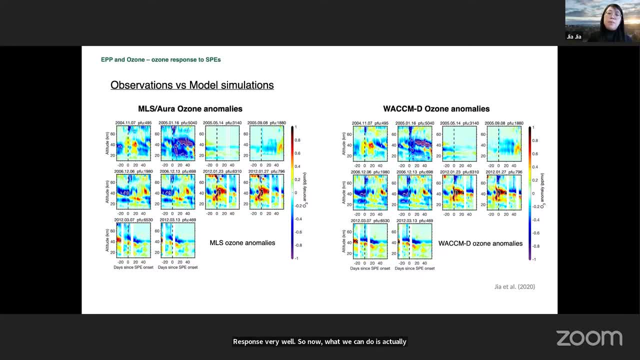 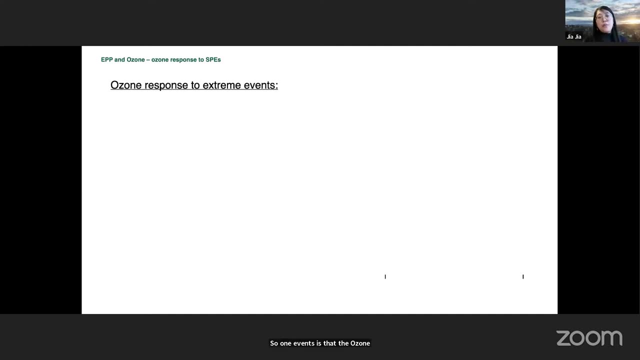 So now what we can do is actually that, since the SP is very sporadic, but now we have a model, so that means that we can- we can play with the model and to test different kind of events. So one event is that the ozone response to the extreme events. 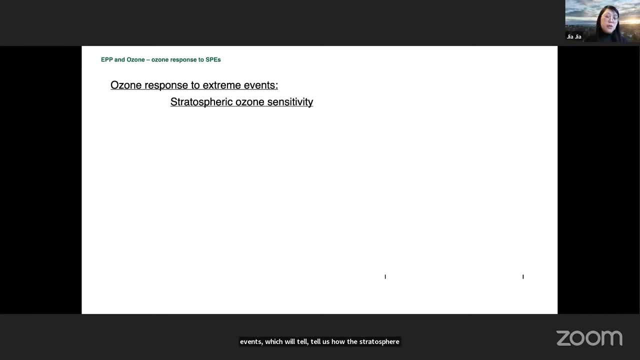 which will tell us how the stratosphere ozone is responding to different events in 2023. So this is a very recent study. There is a paper talking about an event in 2012, July. There is one CME event that happens. So it's a very strong event, but it misses Earth by several days, So it didn't really happen, It didn't hit our atmosphere, but it is the one that is comparable to the one of the biggest events, The one of the biggest observed events. 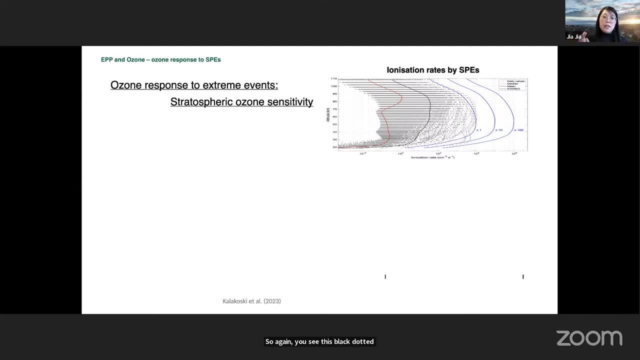 So again you see this: black dotted lines are the SPEs with ionization rate And the black line means the mean ionization rate. happens during the past SPE events And this one is the one that if the event actually hits Earth. So now you see that this event is very comparable to the 2003 Halloween event. 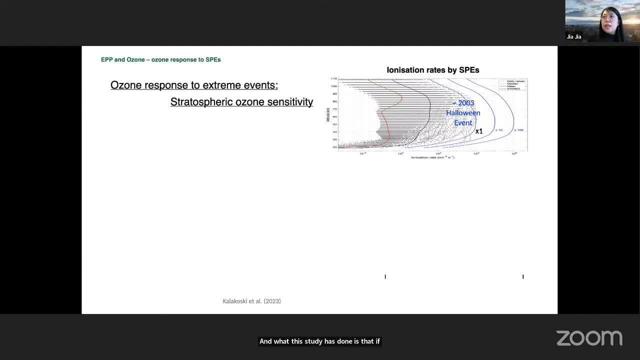 And what this study has done is that if we actually make the ionization larger to 10 times or 100 times, what will happen? So 100 times would mean that is the most strongest solar proton event, with the record which is- I think it's- reported by Ilya Ussotsky. 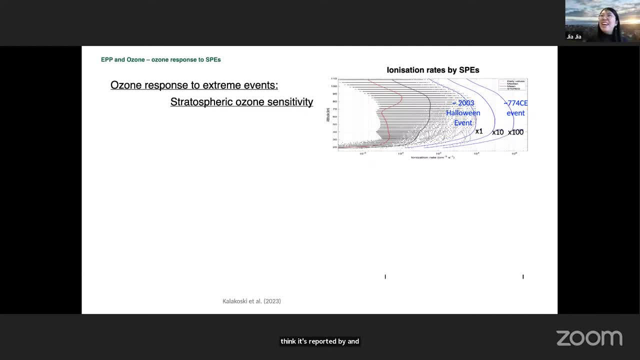 And so I don't remember what, but it was a 774 CE event, So this is a very strong and the most severe SPE event. Now, with the model, we can see how this event responses to the real ionization rate and this very extreme event. 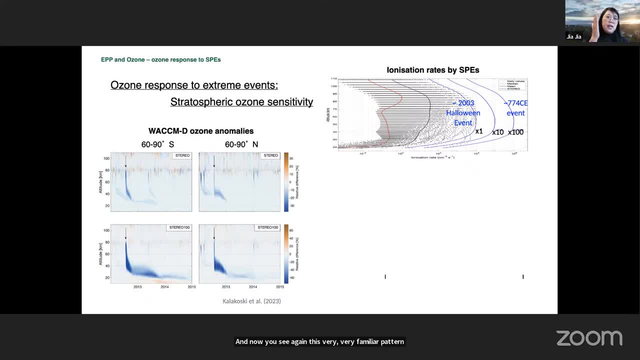 Now you see again this very, very familiar pattern already. The immediate response and the tail response follows it And of course, the severe it is, the bigger the depletion is OK. it's actually not very easy to follow what's going on. 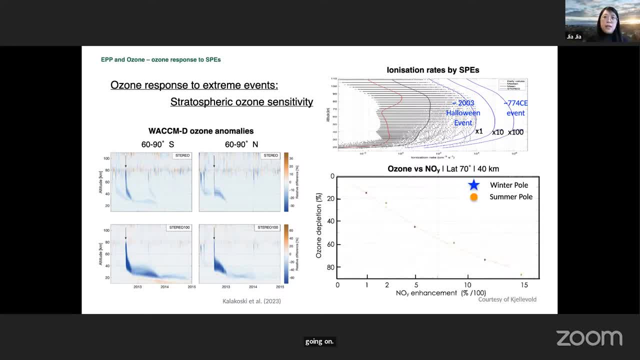 So me and my student, we are working on ozone And so NOx extended family of NOx is called NOy. We're looking at ozone and NOy relationship in this stratosphere layer. So this is a 40 kilometer at latitude. 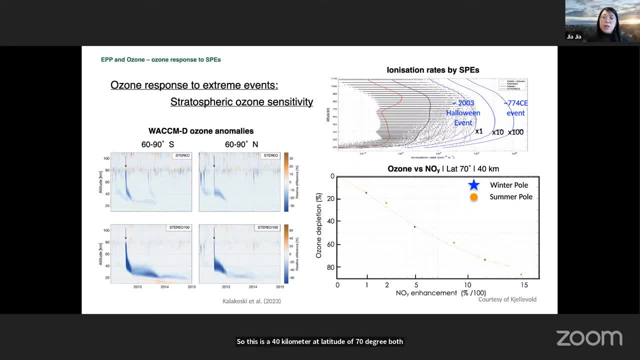 of 70 degree, both in the northern and southern hemisphere. So we have this curve here And if you mark all these events, this is the 2012 event. So 2003 Halloween event, So this is the event itself And this is the ozone level. 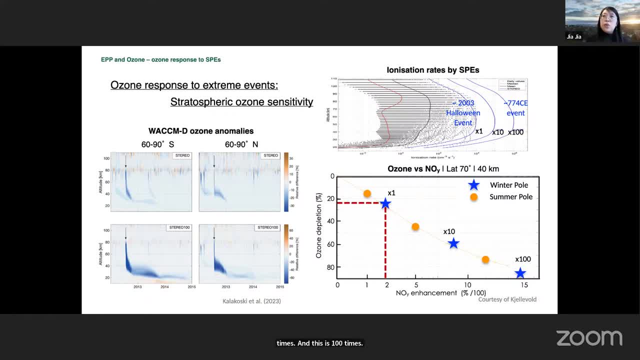 And then this is 10 times and this is 100 times. Now we can see how the ozone depletion would go. So with this event itself it goes to over 20 percent and 20, 25 around, And when it's 10 times it reaches 60 percent. 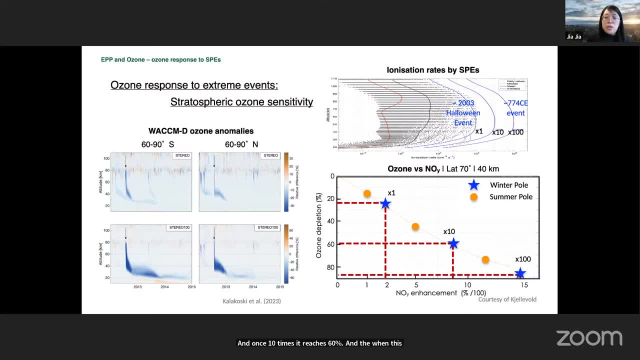 And when this severe event happens, it is almost 90 percent of the ozone in this height being depleted. So we can see that the ozone levels they are much smaller than this. This is because the solar conditions, the sunlit conditions, are different. 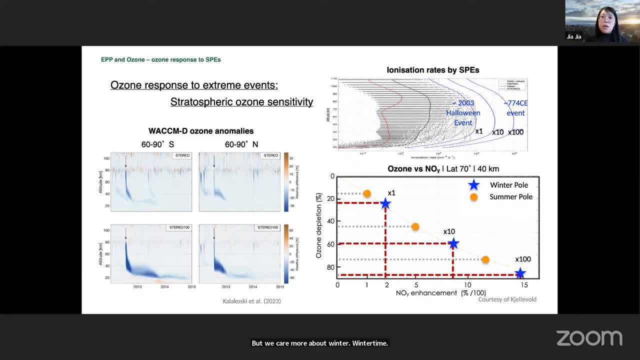 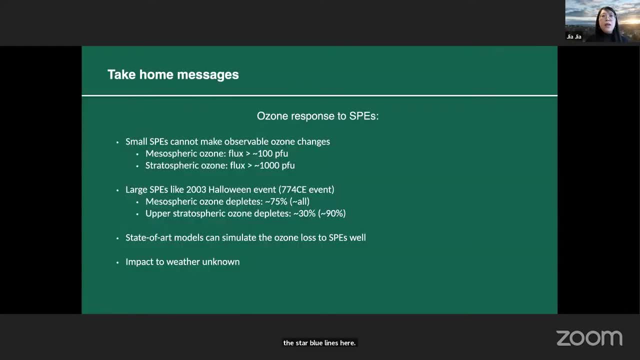 So there is a different balance of ozone, But we care more about wintertime. So those are the star blue lines here. OK, so this is the solar proton event. So just to give you a take home message. these are all the conclusions of what I 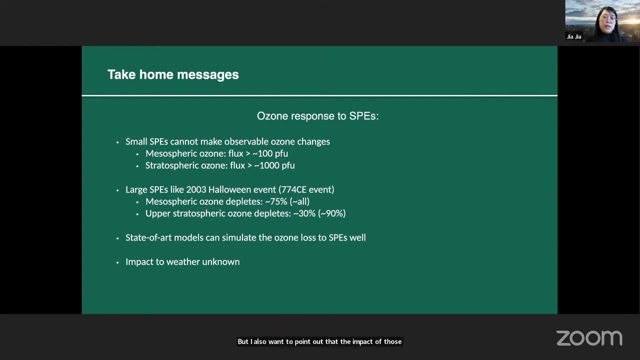 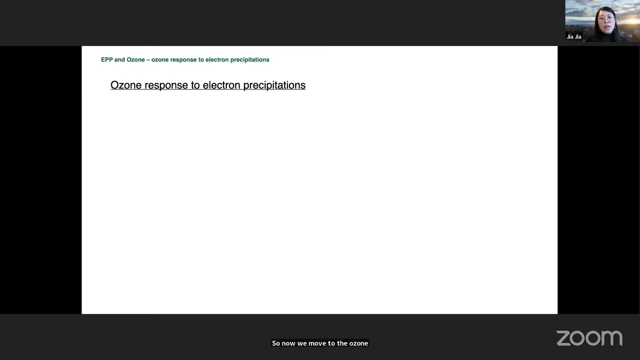 just said, And the impact of those solar proton event to the weather is so far unknown. I don't recall any report telling us what the responses are. So now we move to the ozone response to the electron precipitation. Same story. We will first look at the direct response to this kind of event. 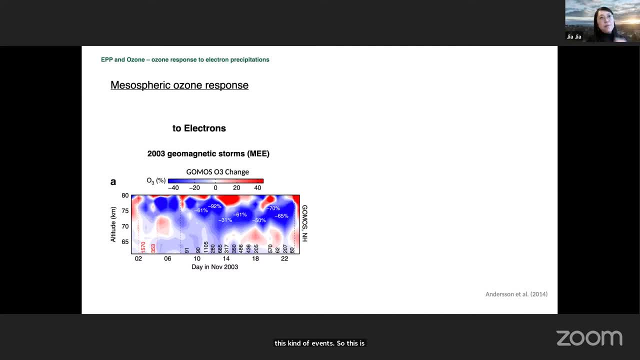 So this is again an event study, So actually follow that 2003.. So this is the ozone response to the solar proton event. There is a huge geomantic storm going on, So this study was the one about geomantic storm. 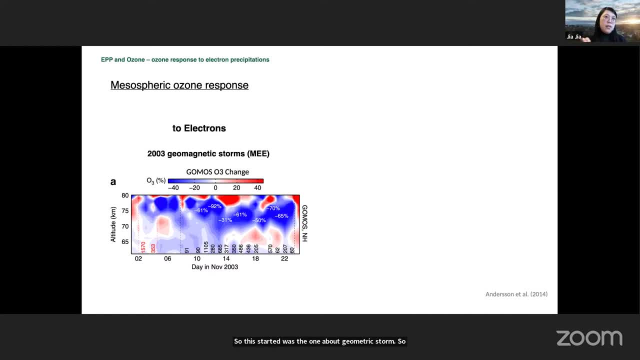 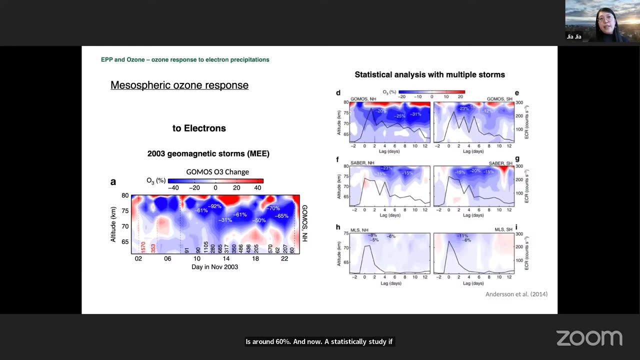 So now you see, the ozone depletion from the satellite observation and the depletion due to the so-called medium energy electrons from the radiation belt is around 60 percent. And now statistically study, if you gather in all this electron event, so the geomantic 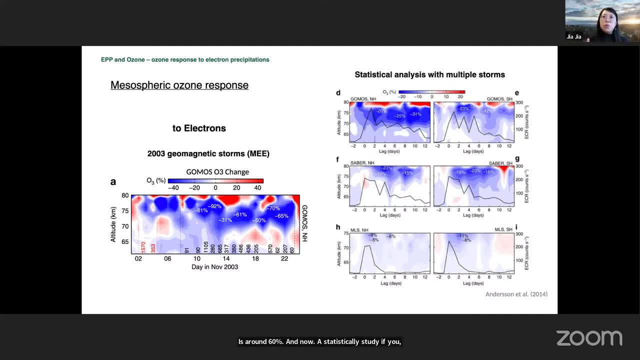 response of the top of the satellite is that you will have different satellites From the different satellite. you will have different results. top is GOMOS, middle is SABRE and below is MRS. Now remember that the satellite has different sensitivity because of the 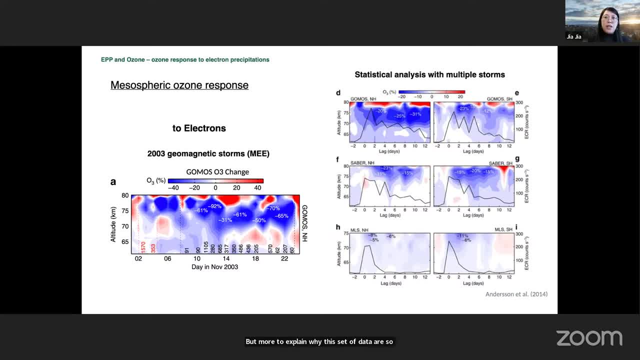 resolution different. But more to explain why this satellite's data are so different is actually that the satellite data measurement has different times of this solar maximum times, while the MRS actually passed it, So it didn't detect the stronger events, But still we don't really know. 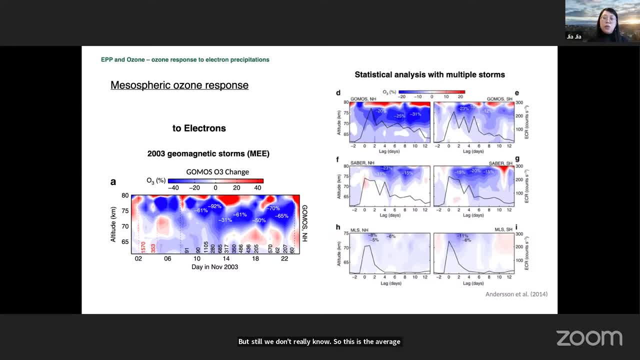 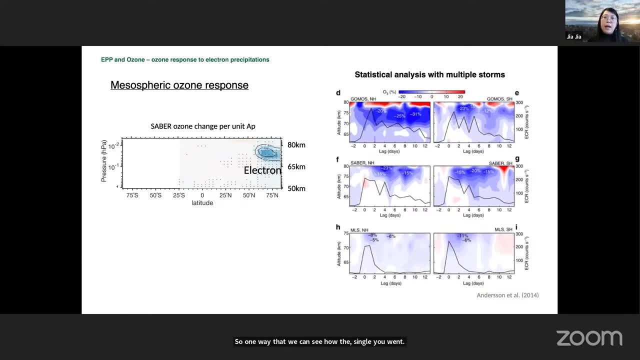 So this is the average. it differs with time. So one way that we can see how the single event will impact on ozone is to look at a relationship between ozone and the AP index, which is reflection of that dramatic storm. Now this is a multiple linear regression. 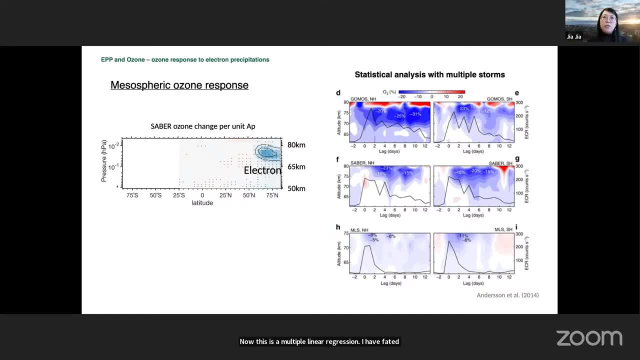 I have fitted it with the AP F10.7, and many other dynamic factors And now you'll see, in the stratosphere we have this blue reaction. That means that ozone reacts like together with AP. The higher AP you have much lower ozone. 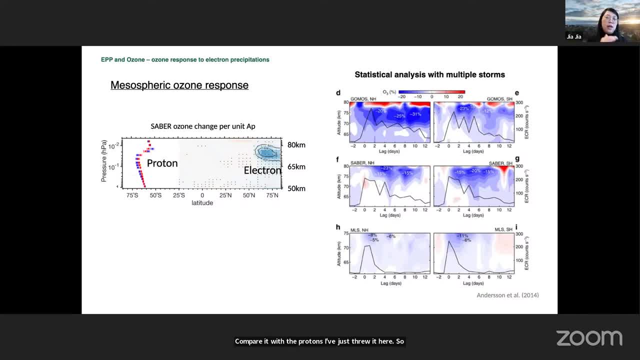 To compare it with the protons, I've just threw it here. So the altitude you see are very similar. So now, with this relationship, we can actually look at how the ozone depletion changes along with the different geometric storm levels. So this is like a preliminary, very rough story. 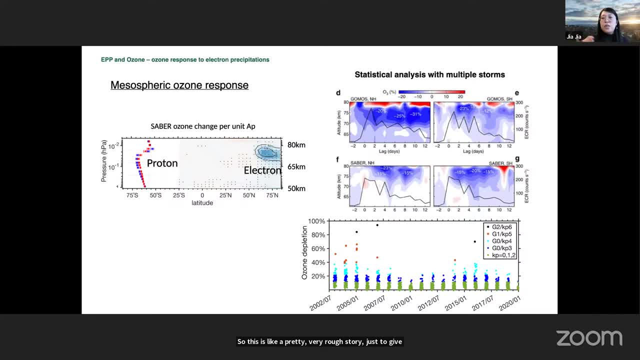 just to give you a concept of how much ozone are depleted. What I do is I just assume ozone doesn't change at all. It has the same value, which is not the truth. It has a seasonal variation, But you will tell immediately, like how the ozone changes are, with different KP values. 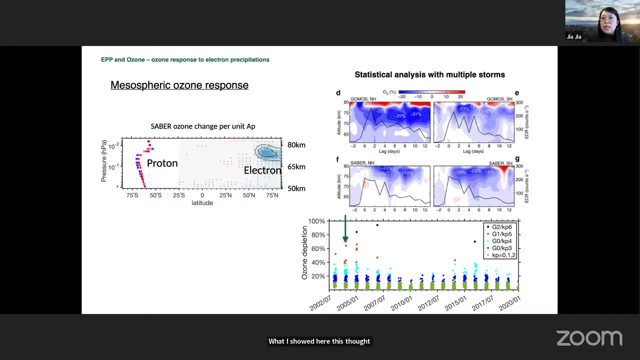 What I showed here, this dot, is this key study I said before, So remember it was around 60% and it is showed here Now you will have a general view as well, Like in average with the active geometric storms. you will see that, yeah, it's around 20%. 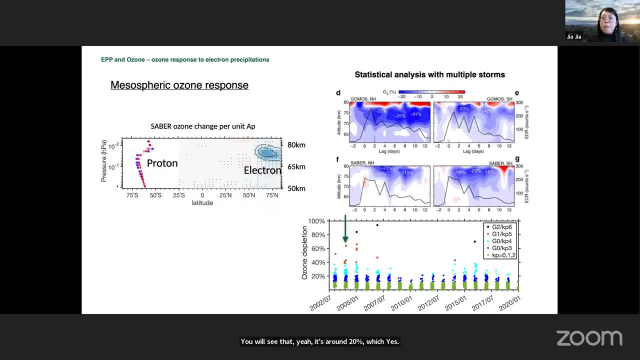 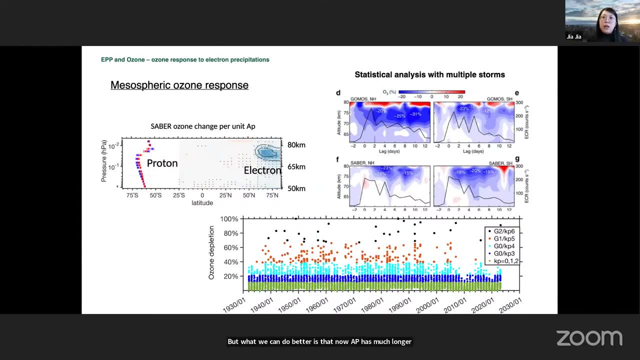 which is consistent with this satellite data. But what we can do better is that now AP has a much longer record history. Now we don't hear about the satellite data, you know. but we have a much longer record history, Now we don't hear about the satellite data. 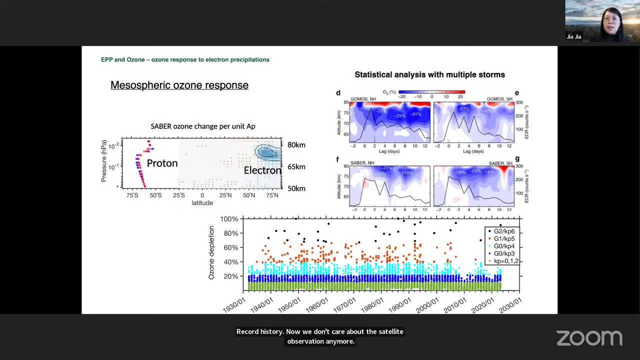 observation anymore. we can really go back to the 1930s. What you immediately realize is right: the solar cycle 24 is a very tiny solar cycle. So before the solar cycles are like they are more active sun and there's more geomantic storms. So now we are not talking about 15 to 20 percent. 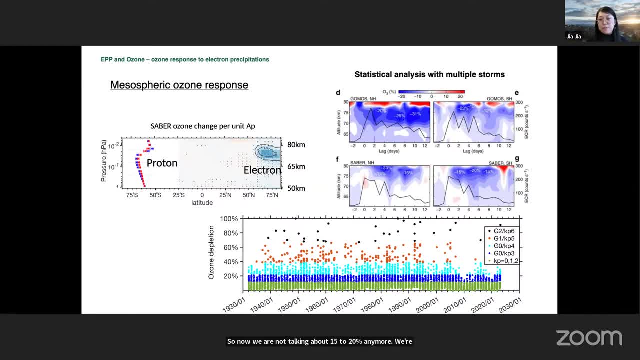 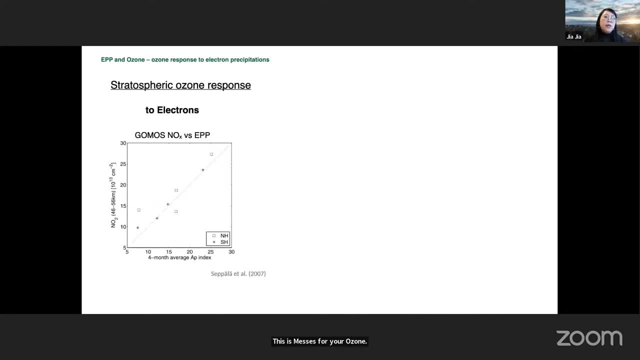 anymore. We're probably talking about 30 to 40 percent. This is mesosphere ozone And, if we go to the stratosphere, ozone, and in 2007,. so this idea about NOx will destroy ozone was already brought up. okay, in the 1970s, But in 2007, there's a paper telling you that the stratosphere 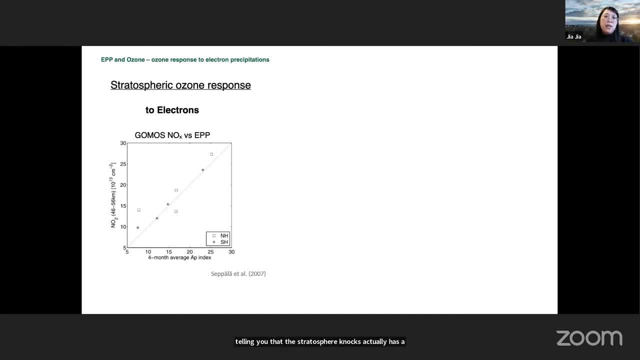 NOx actually has a linear relation with the winter AP condition in average. Now you see that southern hemisphere and northern hemisphere both follows very well with the AP. The more AP, the more NOx. So the stratosphere NOx actually has a linear relation with the winter AP condition. 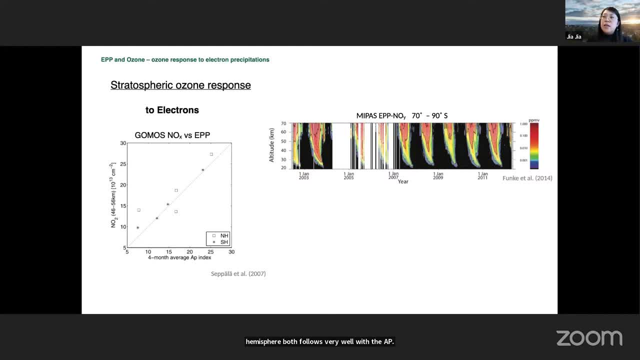 the more NOx Now with the years, in 2014,. we already have a so-called EPP NOy. This is based on the SETTED observation and it tells you how much NOy NOx. quite similar, I would say. 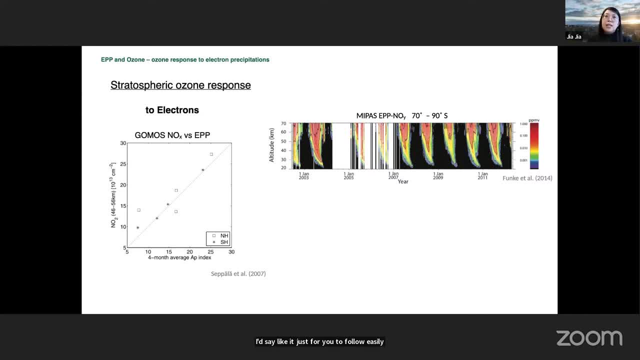 like, just for you to follow easily, that you can see now that it really follows the solar cycle, the 2003,, 2005,. for this solar maximum You have like much, much more NOy being produced and then you have a minimum years. 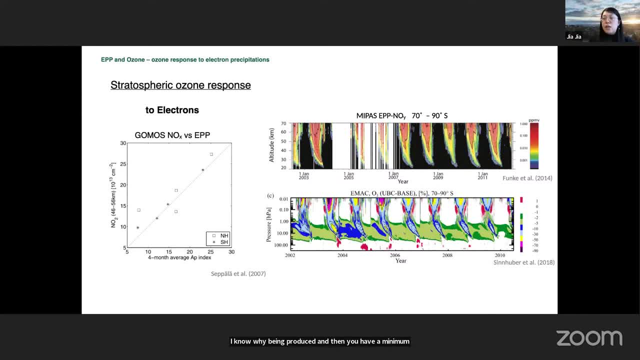 Now with this you can put it into a model until it can tell you how much ozone I depleted. Now, if you look at mesosphere, which is the top part, the upper part of the ozone changes, you will see it's between 10 to 30 percent, But also the solar maximum years you will have 70. 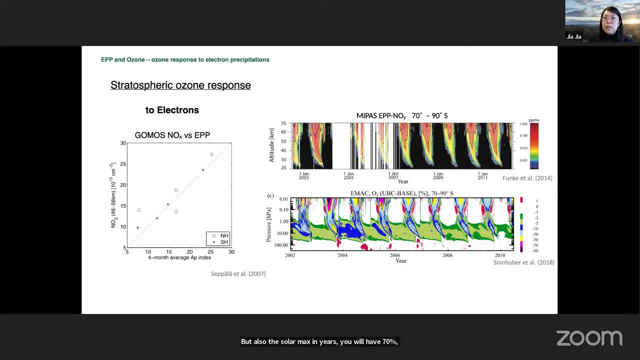 percent, which is consistent And with what I just said. And now, if you look at the stratosphere, you will see that it's a quite similar level of ozone being depleted due to this so-called indirect effect And actually in the solar maximum year around 2003, 2004,. it's actually more than 30 percent. 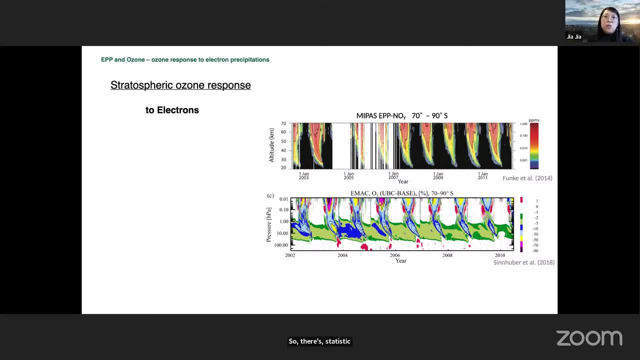 So there's a statistic study as well. So people have just averaged the AP conditions and then also the ozone values coming from the MRS statite and in this winter polar region you will see a statistically strong, significant signal And this tells us it's 12 to 15 percent. 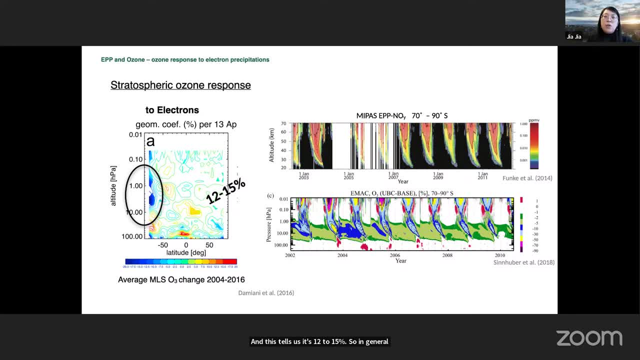 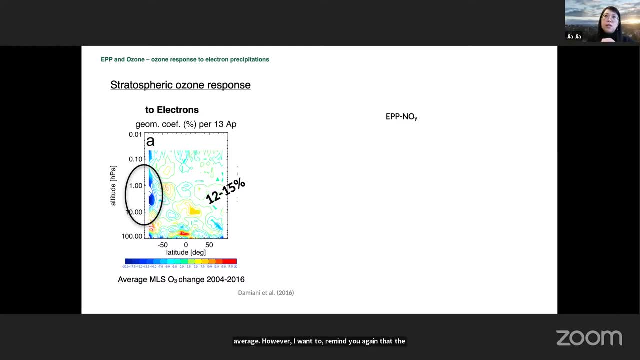 So in general, as an average. However, I want to remind you again that the AP values goes back to the 1930s. So since we know the AP and NOy has kind of this linear relation, you can actually tell how much NOy are produced with the history. Now this is a history line of. 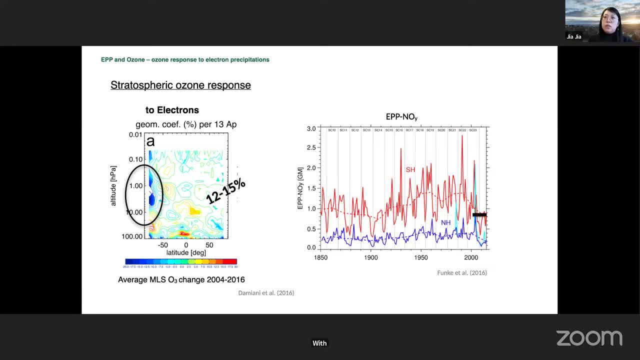 the EPP generated NOy. Now what we have is a satellite observation is at this level. If you go back to solar cycle with 2021, it has a much higher level. So I give a wide guess Now it's. 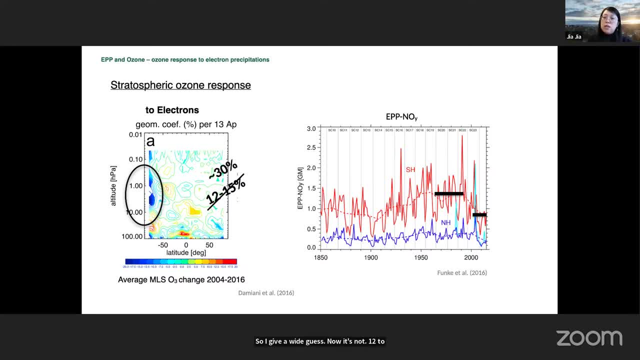 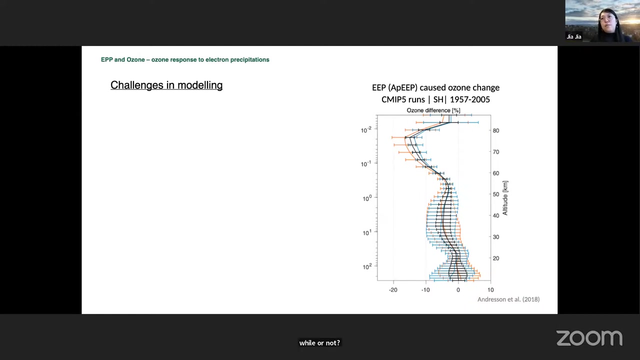 not 12 to 15 percent, but rather more than 30 percent. So now I'd said about solar proton, events have been very well caught by the model. Can we caught this? electron precipitation created ozone, well or not? And the answer is no. So this is a study of the EPP caused the ozone change. 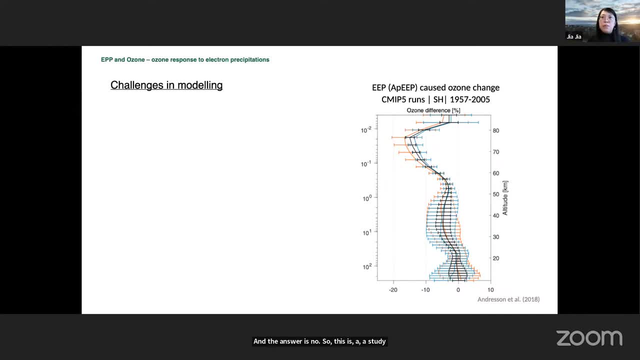 by throwing the ionization rate into a climate model: CMAP5.. Now we have CMAP6 and CMAP7 is on the way. but just to give you an idea, this is a thousand hemisphere and this is like a long-term run. This EPP input is based on so-called APEP. This is created by Max. 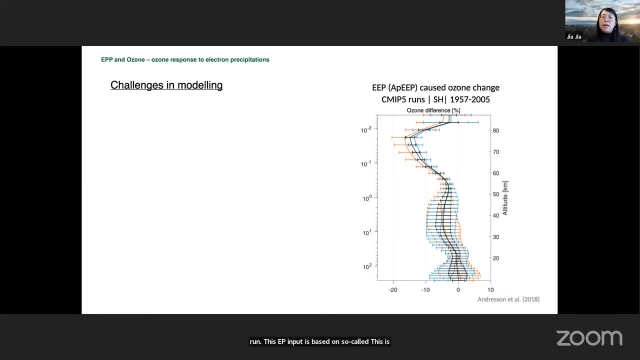 van der Karp based on the AP index, and this is officially used by the current climate model. Now you see that both in the stratosphere and the mesosphere, these values are, uh, much lower than what I have said um the result based on observations. 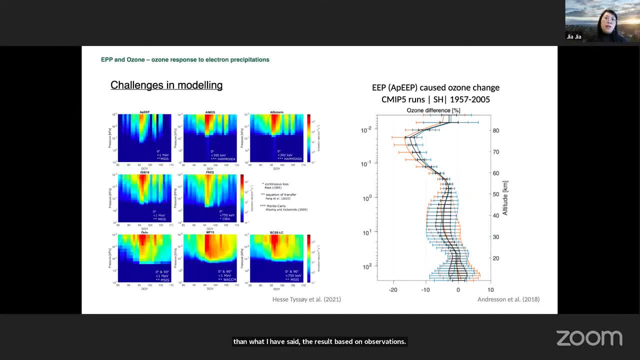 So, uh, why is that? Um, this is because that, um, and this ionization, the AP, APEP and um, they are, uh, indeed, they are, they are uh calculated based on AP, but uh, um, this is. 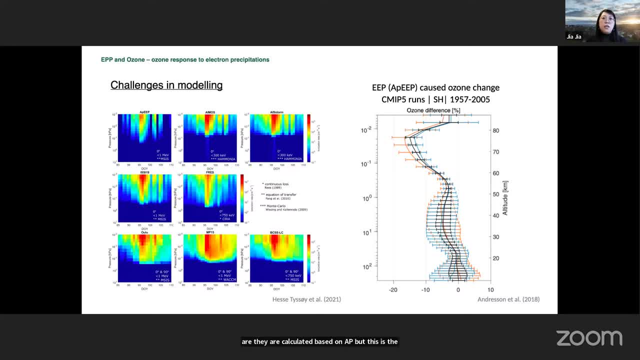 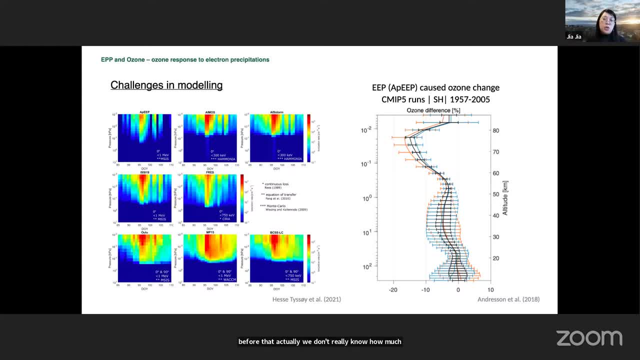 comes into the Loscombe and uh brings these electrons coming into the atmosphere. So we just uh have some um model to calculate that And these are um eight different models and you can see that they give you different ionization rate completely based on how they 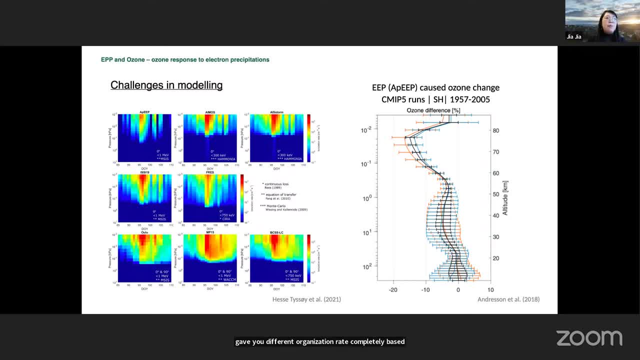 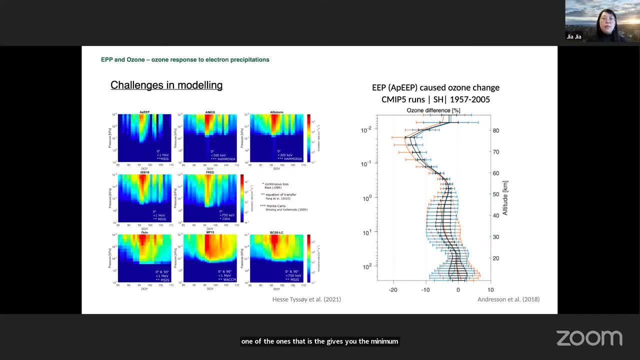 we don't know which is the truth, um, actually, Um, this is one reason. So the ionization rate we put in probably are underestimated, but there's more than that, uh, because we don't really know how the dynamics works, um, how the transport is going on, uh, in the higher layers. So we 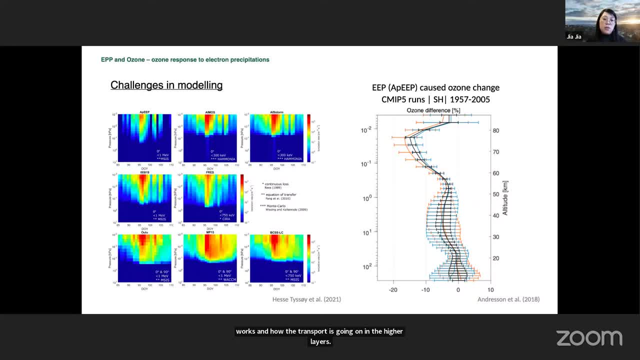 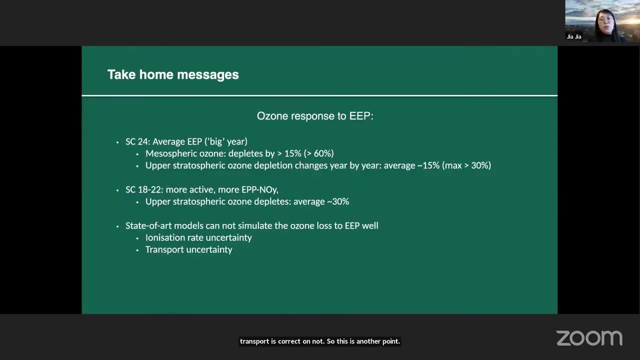 actually don't know, is the transport, uh, the downward transport is correct or not. So this is another point. Um, so with that I have a take home message for the ozone response to the uh electron precipitation. Um, just to give you a quick view. um, I'm not going to repeat. 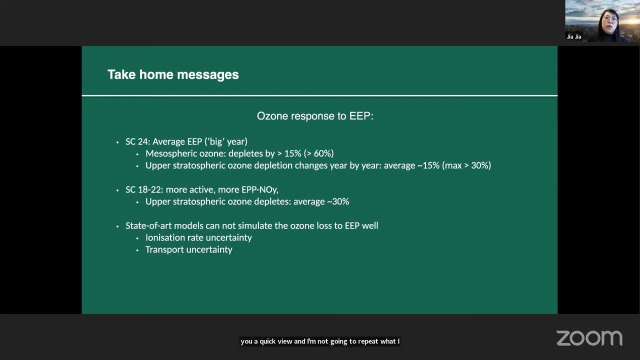 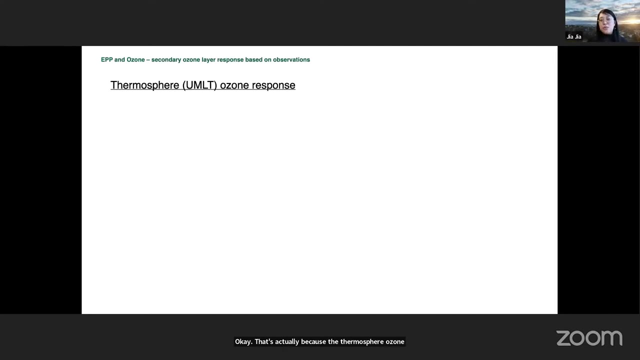 what I have just said. Um, now, uh, we have talked about mesosphere and stratosphere a lot. right, You did notice that I didn't talk about the secondary ozone layer. Um, that's actually because, uh, the thermosphere ozone, which is the secondary ozone layer, are not expected to change. 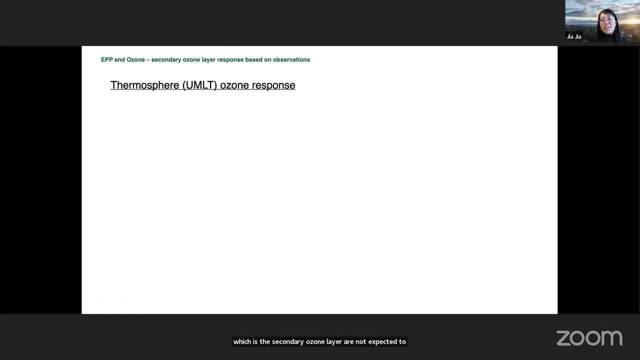 with the, with the EPP? Do you recall that actually EPP changes HOX and NOX? But I said, in the secondary ozone layer ozone is actually more sensitive to atomic hydrogen, which is not really a response. so much with EPP, But, um, but why it still can be related to the energetic 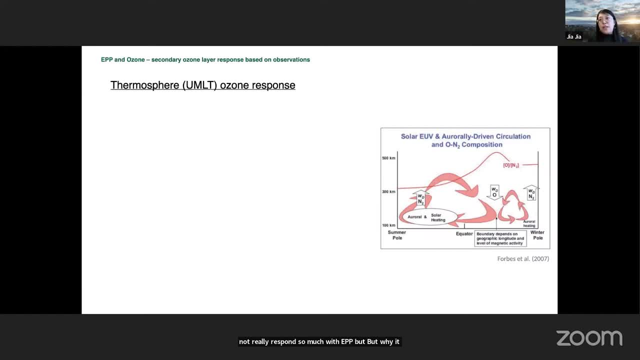 particle precipitation is that the thermosphere circulation will be uh dramatically changed by the, the EPP um, through this uh so-called aurora heating in the polar regions. Uh, it will create this cell that uh uplifting the air in the polar region. 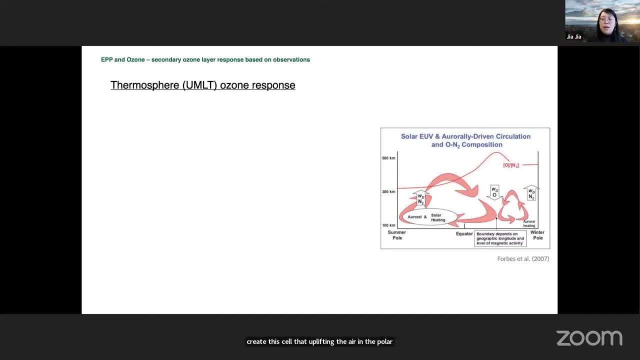 and uh bring it down in this mid-latitude. Uh, so this has been observed with the so-called O-N2 ratio. So we were wondering if ozone would also respond to this circulation change. So I did uh ozone response check with the high APs, the high dramatic storm situation. 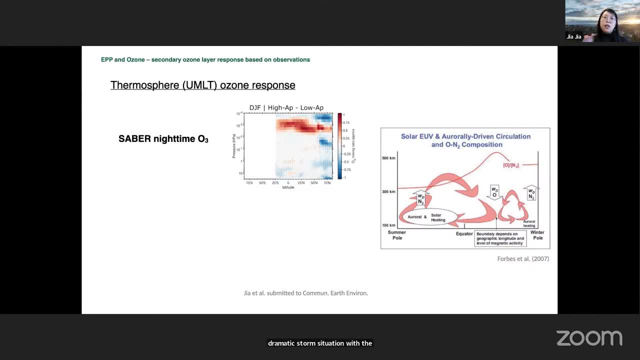 with the no dramatic storm situation. And this is the latitude along the altitude study as well. Now, you see that there's quite some responses going on there. Um but um, there's uh. two things contribute at this height. One is AP, The other thing is actually. 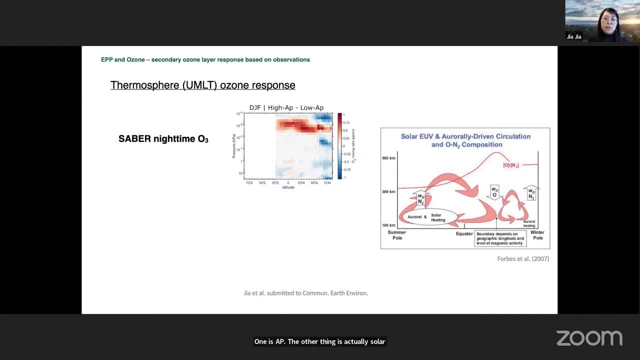 solar irradiance. Uh, the EU way also plays a big role in this ozone uh responses here. So on one side we are pretty sure there's AP uh responses, since this black dots are the significance level, which is a three sigma, which means there's really some significant. 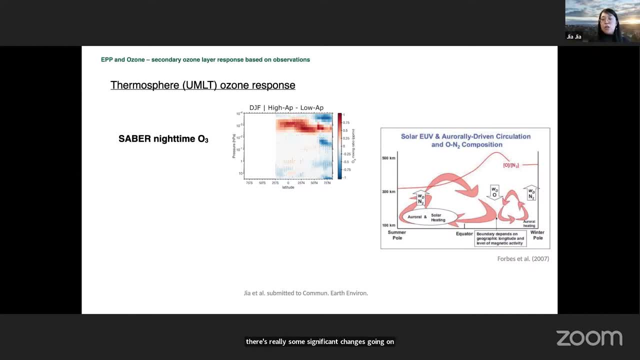 uh changes going on. Um, it is a combination of uh, solar irradiance and this EPP, So I find a way to separate it. Now you are looking at, on the left side is coming from the storm and on the right side is coming from the solar irradiance, the F10.7.. 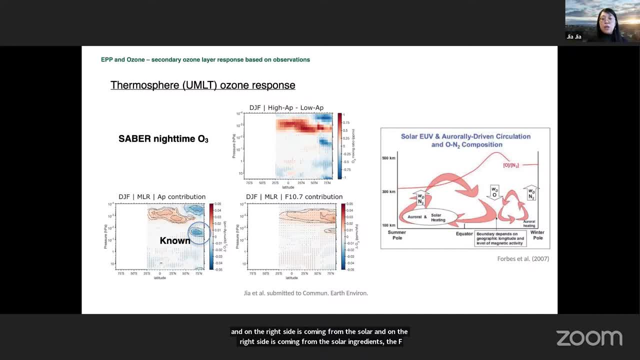 Now, if you look at the AP contribution- and this is what I was talking about- the mass sphere ozone response, this is known. What is unknown is actually here. So you see, there's like: um, we are always talking about the polar region response, but in this layer, 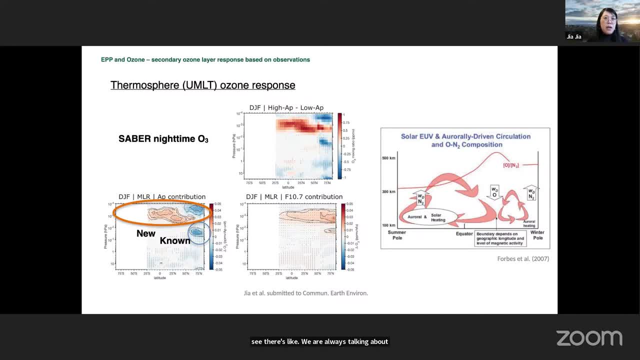 there's actually a global response. Um, so this is the polar region response, but in this layer there's actually a global response. Uh, coming out with this And this uh depletion area in the polar region, immediately we realize this is because of the aurora heating. You have much higher temperature. 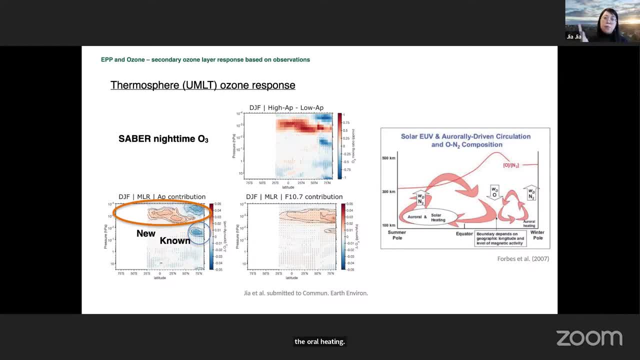 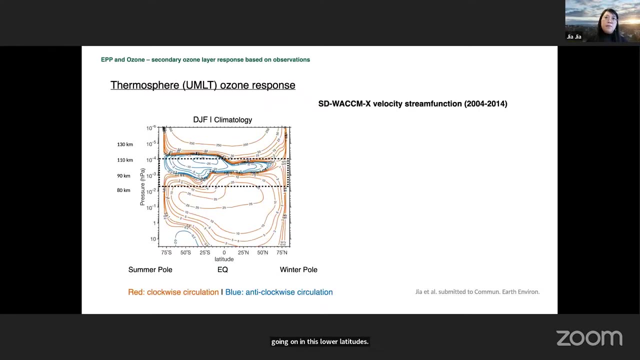 there and ozone, a balance between formation depletion. They actually don't like higher temperature. if a higher temperature, it tends to deplete small. So this is very obvious. Uh, what is not obvious is what's going on in this? uh, lower latitude. So we looked at um how the air circulates. 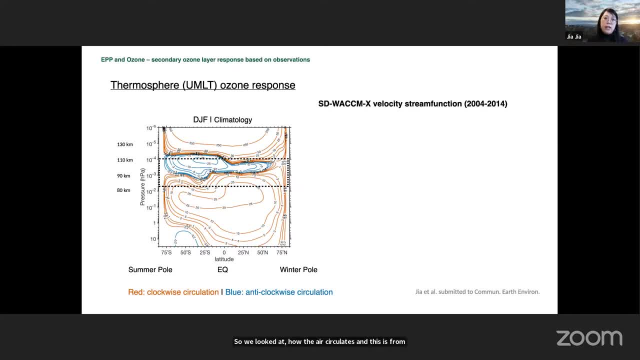 and this is from a model circulation tells you how the air circulates, with the reddish color talking about the clockwise circulation, the blue ones anti-clockwise circulation. So now in the bottom, you see again what I have talked about: this gravity wave dragging summer. 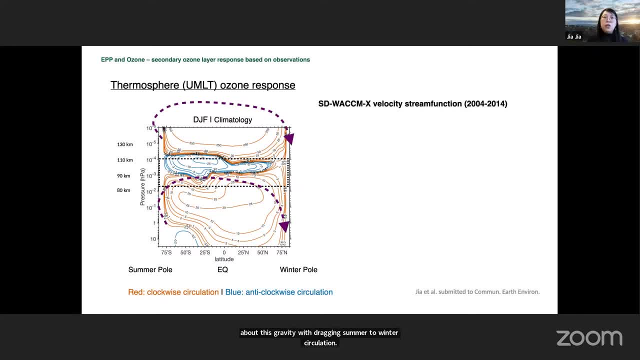 to winter circulation. On the top is a solar uv dragging from summer to winter pole and then you have this reversed part in the middle. Now, when you have a high solar dramatic storm, then you have this polar region. you see there's a blue circle suddenly appears there. that is caused by 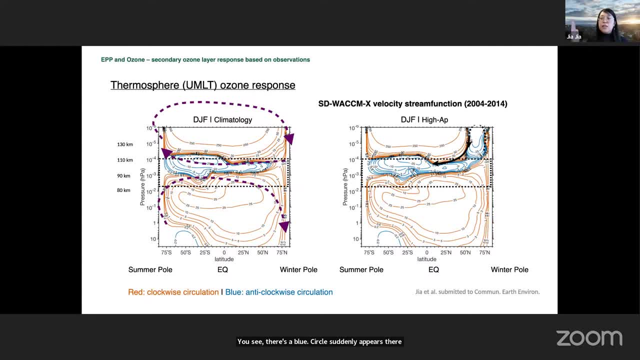 aurora heating And on the very high latitude, around 75 kilometer, you see there's upwelling going on, and that's what we know. and then in the around 50 degree in the north, you have this downwelling coming down. Now what is interesting? 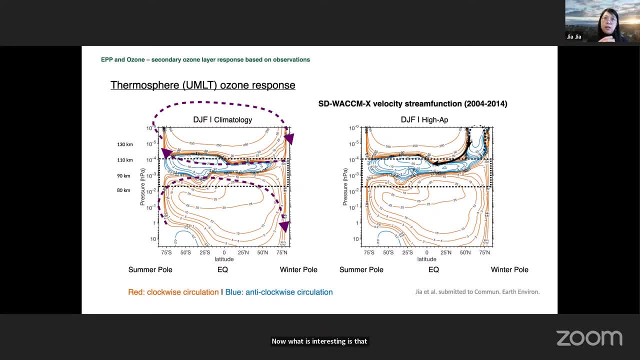 is that this cell is actually connected with the background cell. that kind of like opens a tunnel to transport the airs between the polar region and the low height. So our question is: is ozone maybe another indicator for this layers transport? Yeah, probably. Let's back to this temperature. 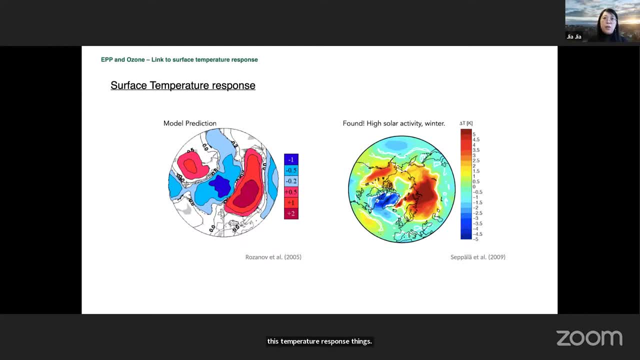 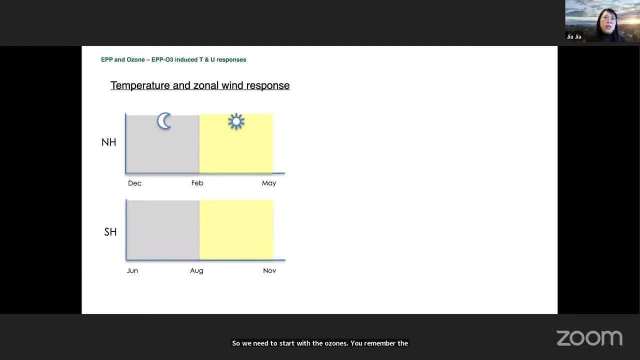 response things. So this is all the starting about why ozone matters, right, And you may wonder what's going on. What's the link Why the ozone matters makes this change. So we need to start with the ozones. You remember the radiative forcing, and then we start to, and then we have 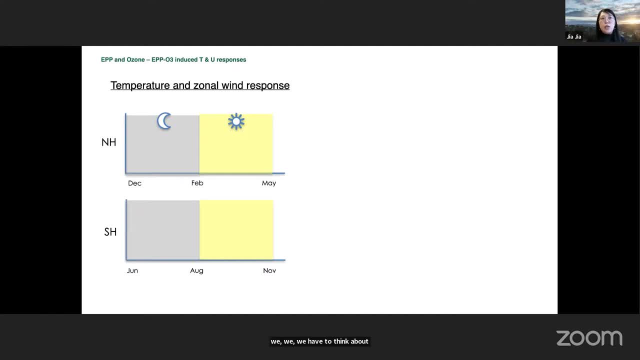 to think about this. polar vortex conditions when the transport also plays a role. So, in the northern hemisphere, now you have this winter dark month, and then the sun start to shine. In the southern hemisphere this is the same story. However, the polar vortex, which is the strong, the wind, 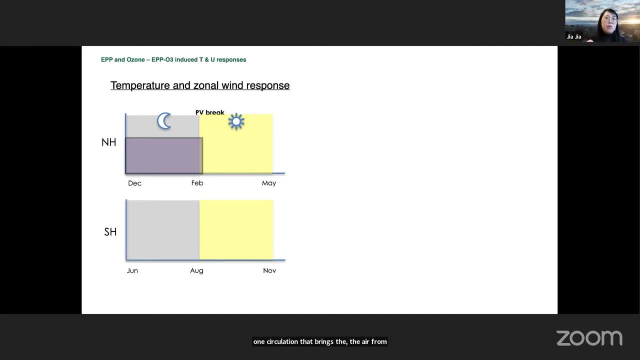 circulation that brings the air from atmosphere down. they are different. In the northern hemisphere, the polar vortex breaks in February, while it's summer hemisphere it breaks in November, which means it covers both. the dark month is also the. the sunny month is, So what? 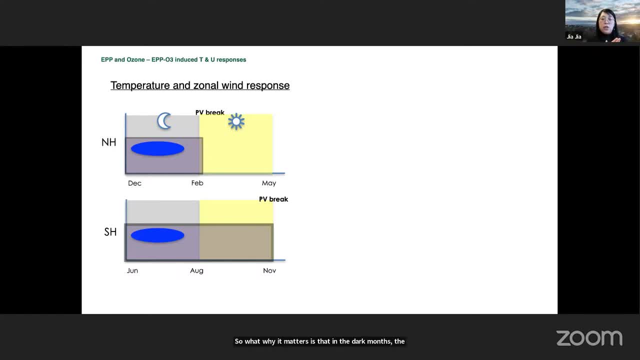 why it matters is that in the dark month is the ozone more like a cooling engine, and when you have ozone that is eating away, you have a relative heating, while in this sunlit conditions the sun actually works, the the ozone actually works as a heating engine. so that's completely different story, which makes this topic very complicated. but since we 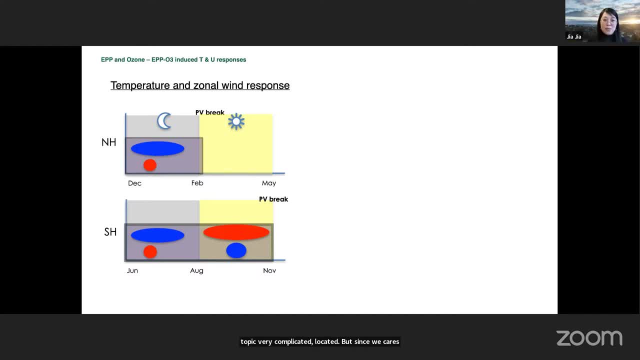 cares about the arctic region because this is where we are, we are living and we care more about this surface temperature change, which is also reported. so we are talking about this scenario, so there's a lot of studies taking into this care and then look at how the atmosphere responses. 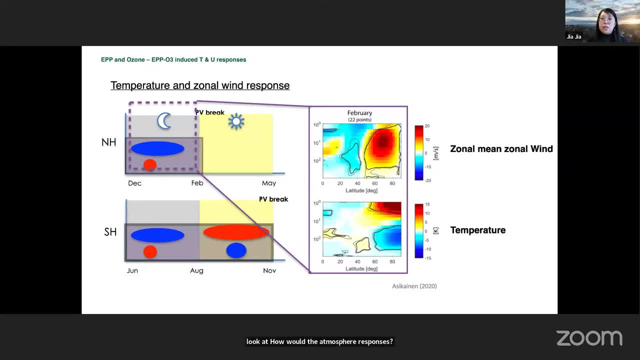 here i show a temperature and wind responses. in the lower part you see the temperature response, and this part is when the ozone is eaten away by the epp and then you will have the so-called radiative warming. but you will also notice that's not only the layer. 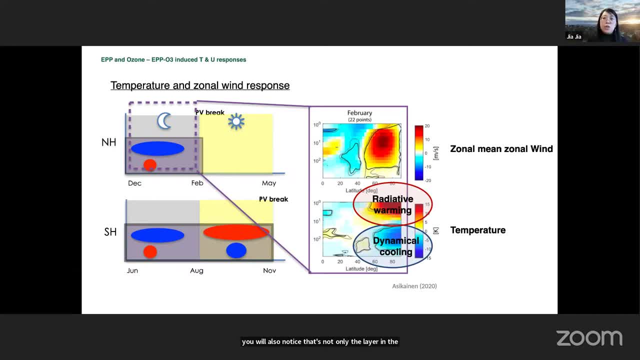 you will also notice that's not only the layer. you will also notice that's not only the layer. in the lower part there is a so-called dynamic cooling which also reacts to the epp and this. altogether it forms in the top part. you will see that this red color is the enhancement of this. 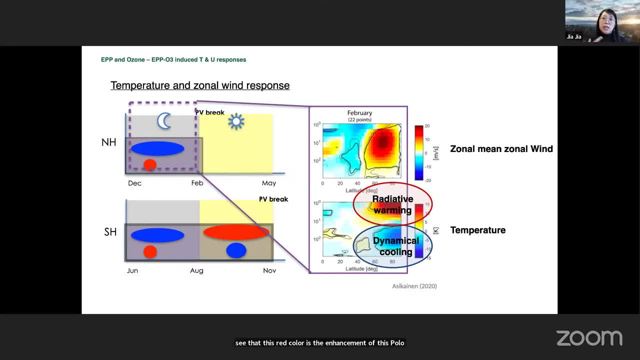 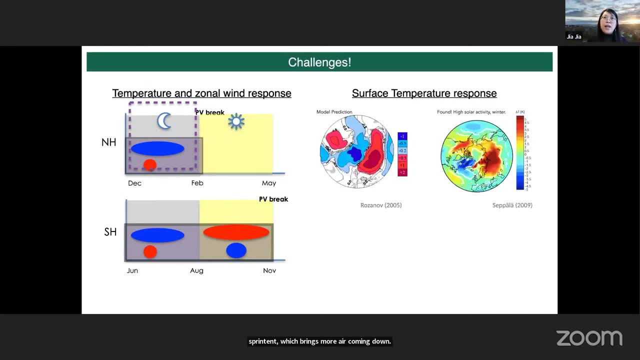 polar vortex, which means the the polar vortex is strengthened, which brings more air coming down. but do we understand what is going on between those wind and temperature changes and the surface temperature changes changes? the answer is no. so the mechanics of these responses are how they are linking together. 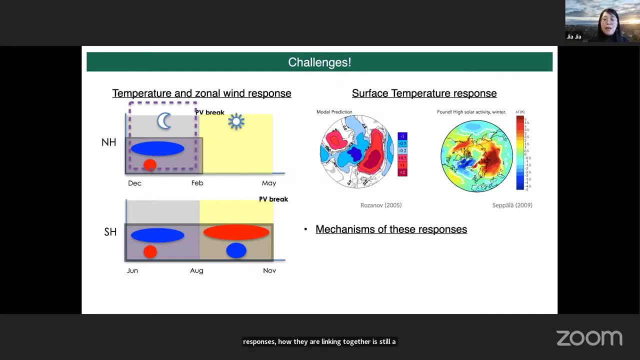 is still a topic that we are really working on on the other side side, since the climate models underestimate and know why it doesn't really reproduce how the climate impact would would be in reality. so there's a lot of things we need to do. we need to correct this loscon issue to get the 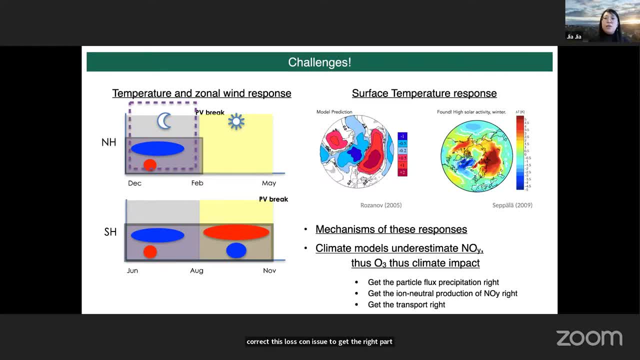 right population and we need to correct this loss con issue to get the right population and we need to of fluxes into the atmosphere and then we need to get the transport of the atmosphere model right. um, these are the things, so i don't know how much time i have. maybe have exceeded the 45 minutes. 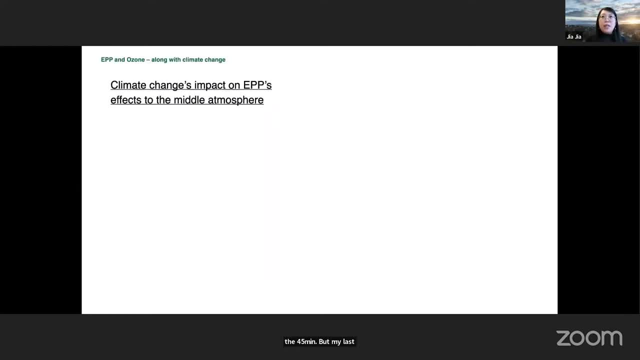 um, but my last side is: uh, my last point is actually: uh, we all know there is a climate change going on, right the tipping point, and so many extreme events happening right now. so how would the climate changes impact on this epp's effect to our atmosphere? um, here's a study. 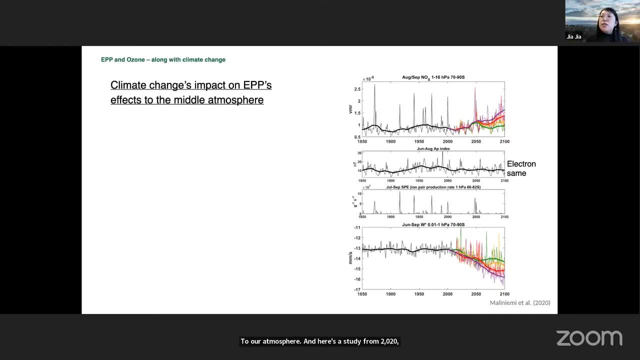 from 2020, which tells us that if you keep the electron and protons the same on the bottom panel is actually this downward transport of the air. so you will see that with the climate change and the so-called boradox, and circulation accelerate, which brings more mass sphere. 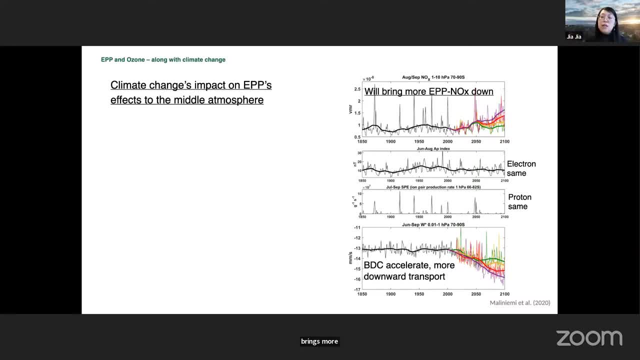 air down into the stratosphere and this means on the top part, is the nox response is that it will bring more epp generated nox down to this critical ozone layer area, which will change the ozone. um. so very recently- this is a october, november 2023- there's a report of ozone trend in the 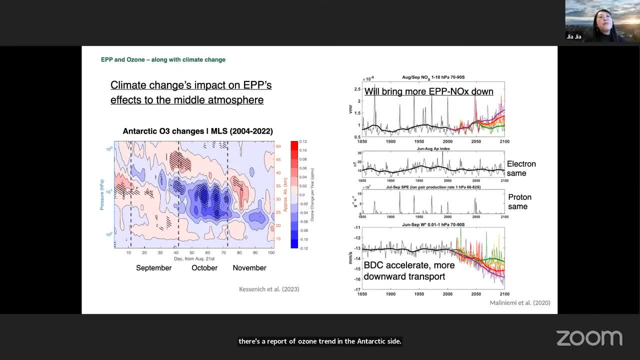 antarctic side. so this ozone hole study, sorry, and this is using the satellite data. again, this is um, um and it gives you how the ozone changes on different days. uh, along the winter time, in the september and or also in the most of the areas. you see that and this is the effect of the motor. 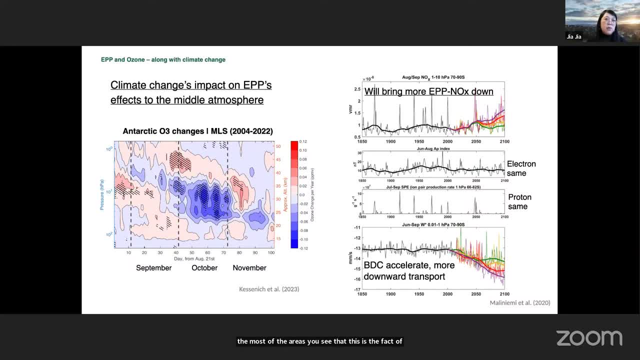 motor protocol, that we have less chlorine and this- the ozone hole is recovering. however, what is weird is, in october, they found ozone depletion still going on, so this is, uh, actually very surprising. so what they have found out is that these are due to the dynamic changes in the mass sphere that 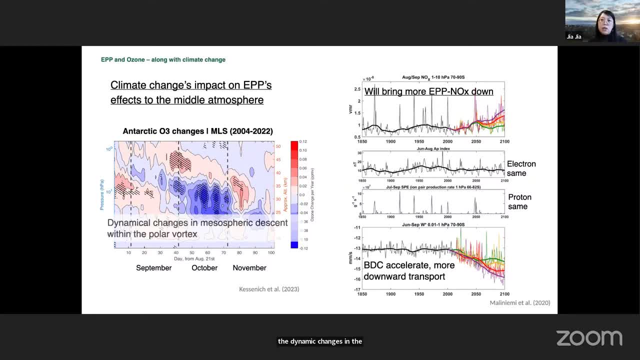 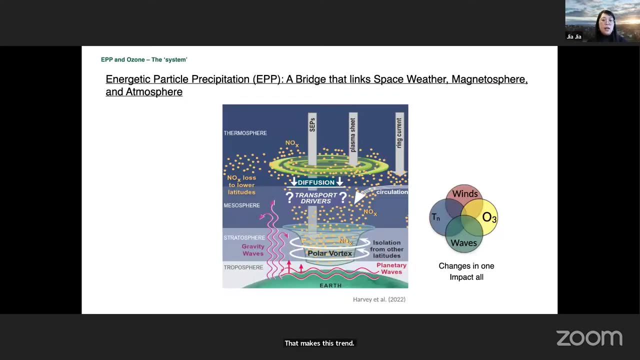 descend within the polar vortex. this trend is has been going on, so the descending is getting stronger and the ozone happens uh in the october- reaches the stratosphere area. that makes this trend so um. i think with that i have uh come to the end of this talk, so this is a complex story of atmosphere. 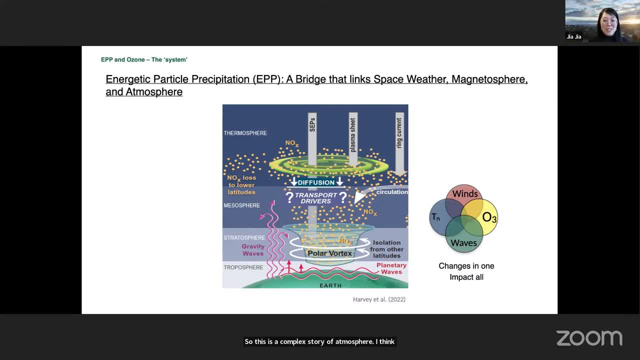 i think you're. i hope you are still following. i mean, it's quite uh, quite a pile going on there, um, but ozone is very important and uh, and this epp is like a gigantic nature uh experiment that the the nature has gave us that we have a chance to use in this epp and atmosphere response. 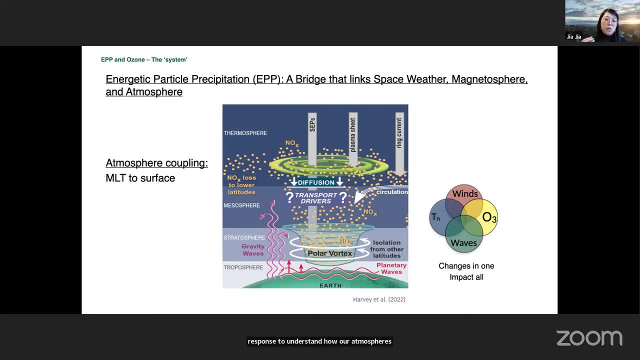 to understand how our atmosphere is coupling from the upper uh layer until the surface, and then also um. it reminds us that compositions like ozone, uh, co2 are the indicator, uh sorry- co and so on are the indicators of transport. this will help us to understand what's going on with the transport which 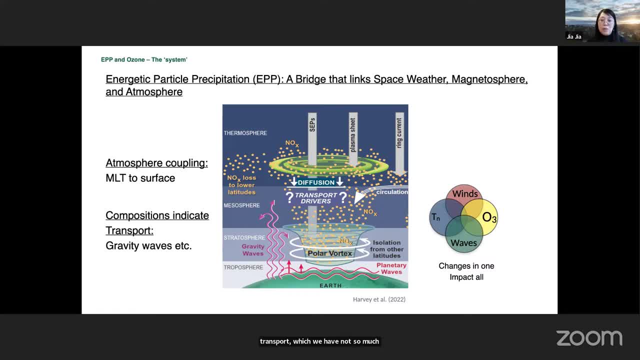 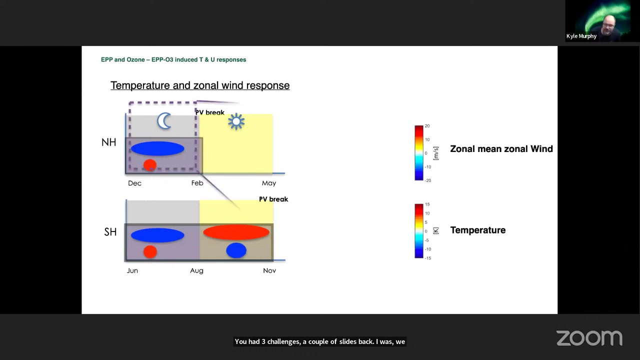 we have, um, not so much information, especially in the higher part of the atmosphere. with that, thank you for your attention. all right, thank you, john, for a really, really cool talk. um, i do have a quick question. uh, you had three challenges. a couple of slides back. I will say we do have applause in the audience, just to point that out. 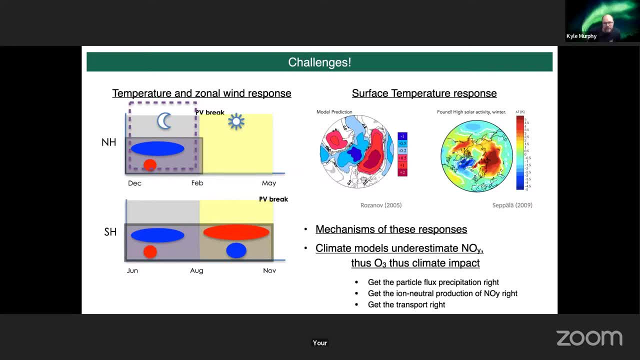 Your challenges. Yeah, So the first two here I see as being tractable. The third one I see as being a little bit more difficult. How do you see the third challenge there being solved? What's required for that? The transport. Yes, So the transport challenge is actually that we count. 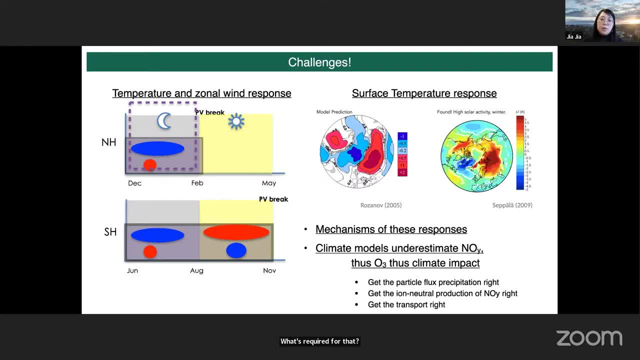 in the model that we So, first of all in the observation in the higher part, so in the lower part until 50 kilometer, we have quite some wind data to tell us what's going on in the atmosphere About 50 kilometer. we don't know so much. There's simply not so many observations going on. 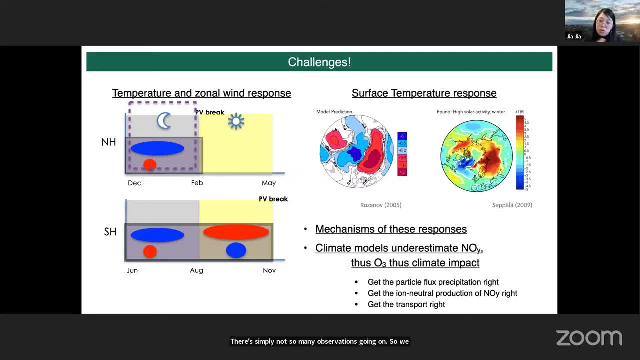 So we don't have an observation for us to cross-checking with the model. So what the model do is normally a free run, And there's one thing is the importance of gravity wave there. So currently the model is using parametrization of a gravity wave And that's not good enough so far. So that's why I was talking. 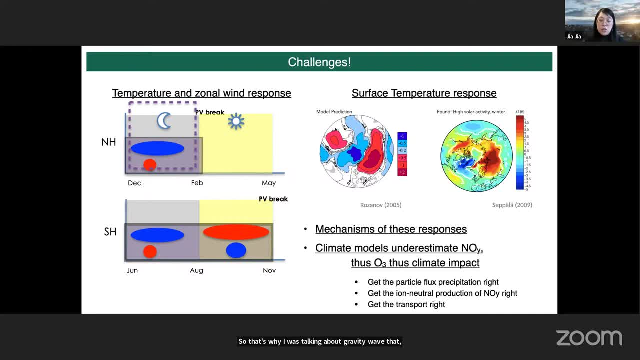 about gravity wave, that if you have a better understanding of what's going on, then probably there's more downward transport in the polar region. So currently we understand is that in mass sphere transport is this diffusion, but probably there's more stronger things going on. Yep, That makes total sense. I was thinking models As a magnetosphere. 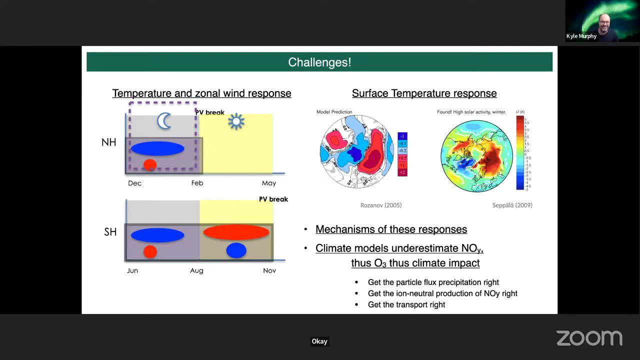 physicist, I forgot you can measure wind, which is silly. Yeah, we actually don't know so much. That's why this thermosphere ozone thing is kind of like for me it's very interesting, Yeah. So, regarding the first one, this does come back to more magnetospheric. 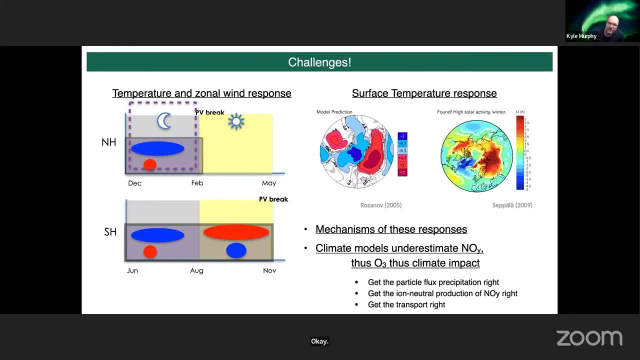 love them. the demands of shrimp, the incentives of life is, I would argue. I'm a sathing. I like the words a lot fits her. deserve, with relatable introduction of is natural and human activity, And directly as a fan of 승, I can see that it's a little bit. 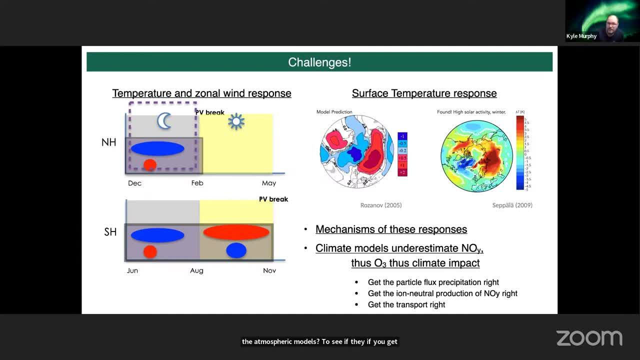 beyond guides, because it's sort of collecting vine kn. Yeah, I would agree. You can't predict all ones anymore, Right, Yeah, Sorry to interrupt you. Yeah, Yeah, hot topic that many of my colleagues is working on, so I'm not directly involved in it, but I can. 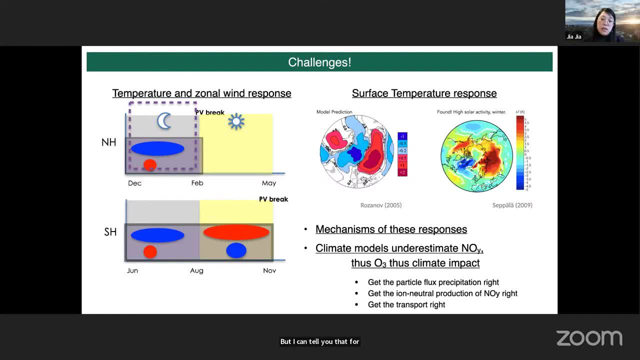 tell you that, for instance, we of course want to. with more observation, we can actually better checking the models. so, for instance, there's an APAP which I was talking about putting into the climate model, and there's an APAP version 2 coming and there's effort going on and then for 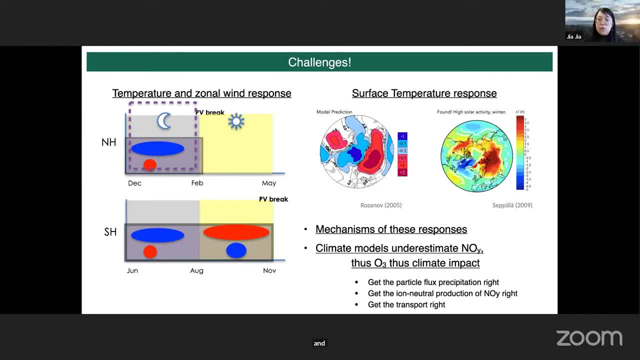 all the other models. I have showed you the eight models and of course, they have their own development as well. it's cool. well, I think that's all we have today. Thank you again for giving a talk today. I hope, for those that are able to see the eclipse, that they're able.